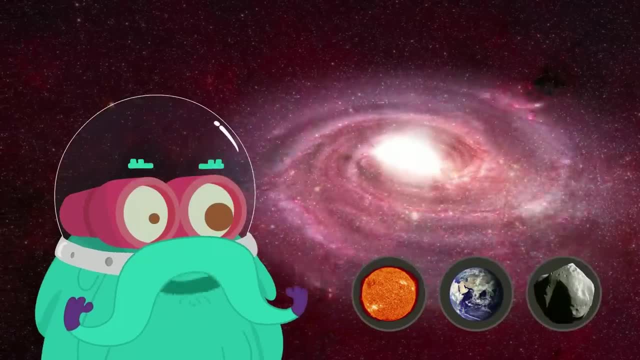 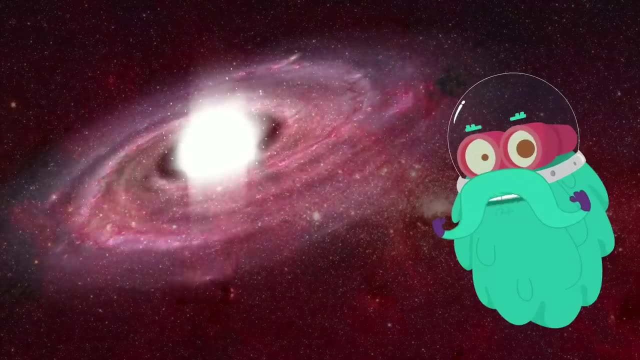 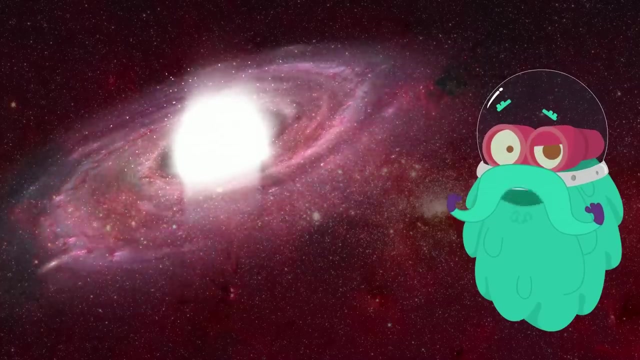 from which the sun, planets and other solar system bodies like asteroids, meteors and moons were formed. Okay, so let's now continue from where we left off. When the spinning slowed down, the centre of the solar nebula became hotter and denser. 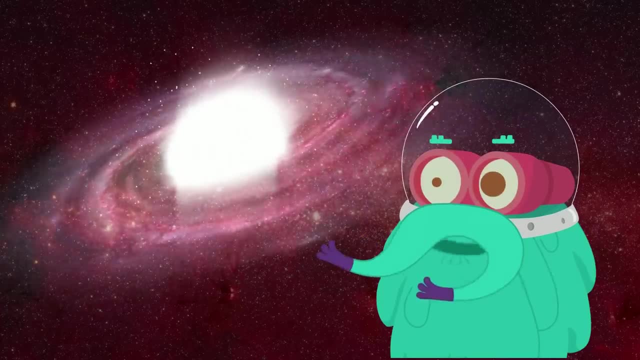 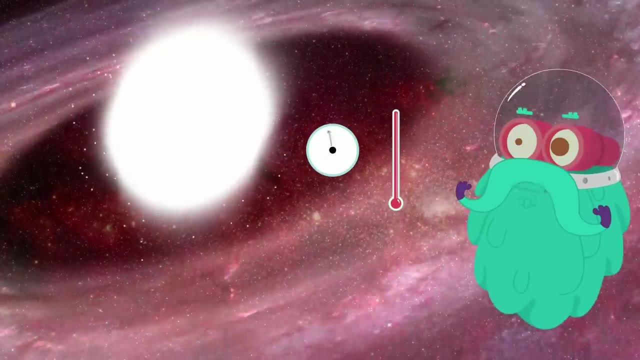 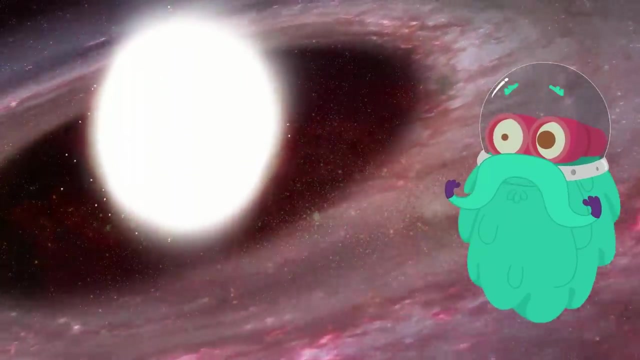 which was surrounded by a disk of gas and dust that was cool at the edges. At the heart of the nebula there was a ball of hydrogen gas whose pressure and temperature became quite huge and the particles began to fuse together. There it was a new powerful star coming into being. 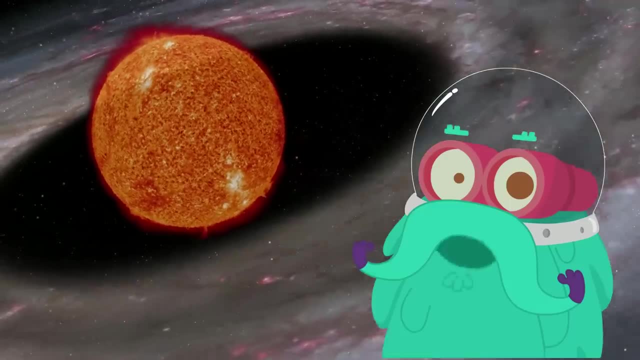 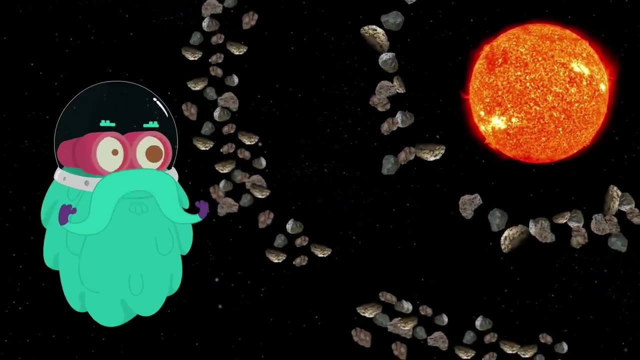 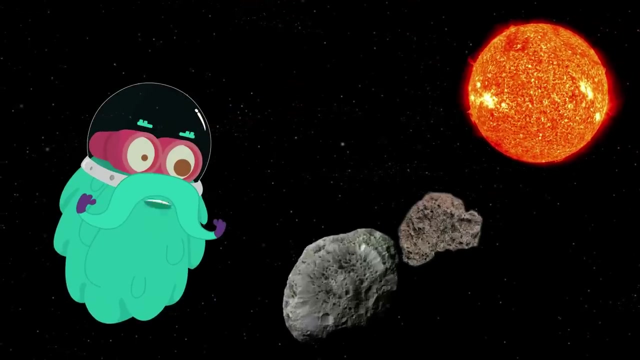 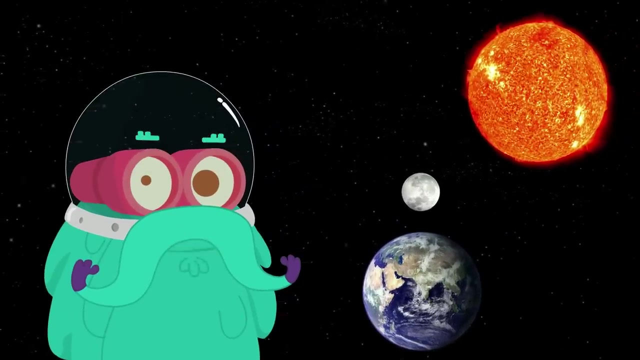 Yes, that was our sun shining like a fiery ball. There were infinite number of particles that began to stick together and formed clumps. Some clumps got bigger and bigger and bigger, forming planets and moons. Aha, so now you know how the planets were born, isn't it? 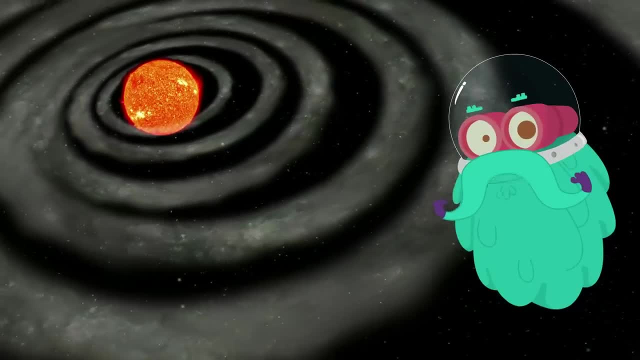 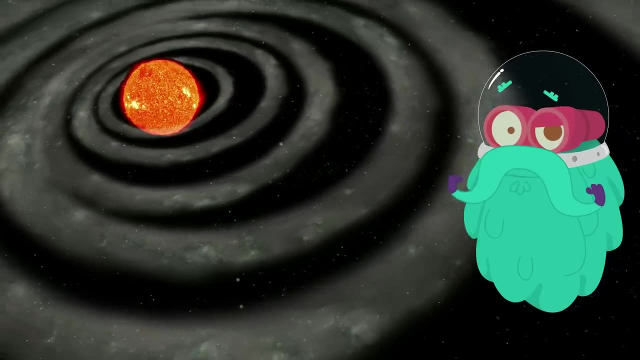 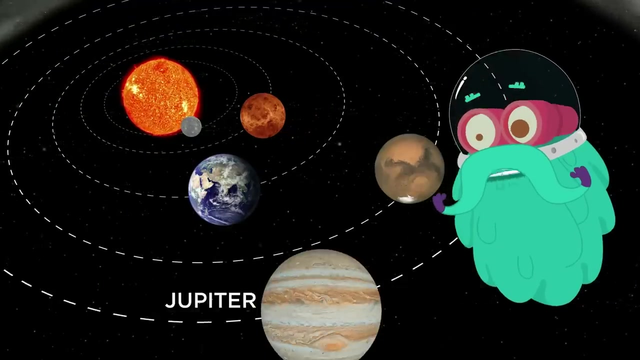 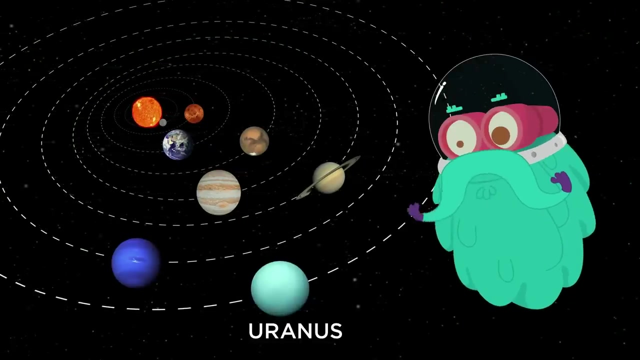 It is also believed that since the centre of the solar nebula was hot, it was easier for some planets to form in there, like Mercury, Venus, Earth, Mars and Jupiter. The rest of the cold planets, like Saturn, Neptune, Uranus, etc. were formed at the edges. 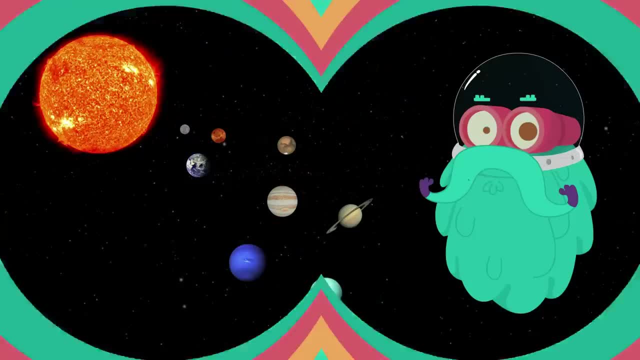 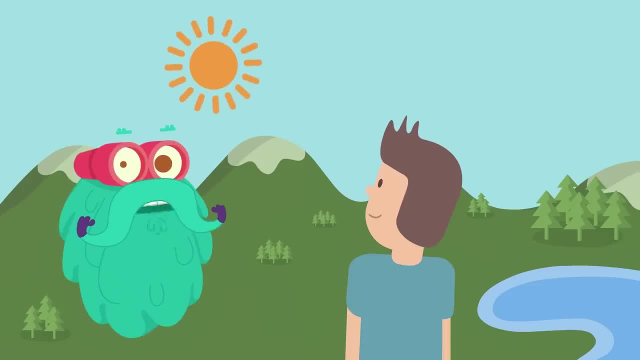 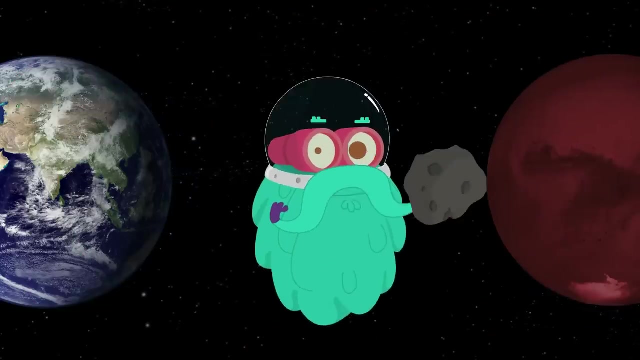 Trivia time. Did you know that the sun takes up 99% of the solar system's mass? This means that we are technically living inside the atmosphere of the sun. The rocks that belong to Mars have been found on Earth, And guess what? We didn't bring them here. 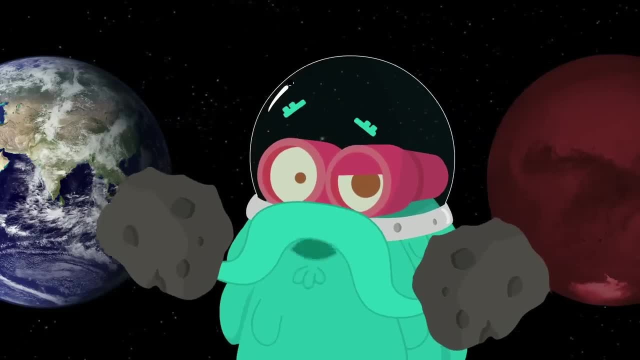 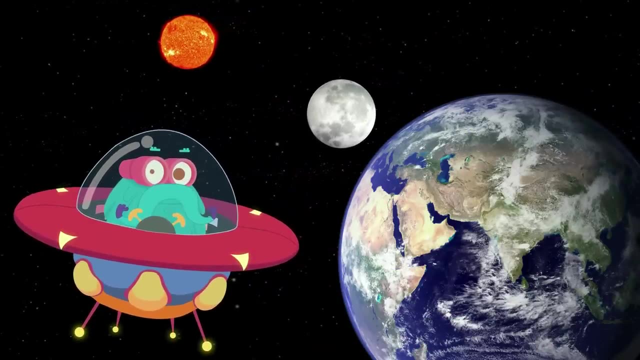 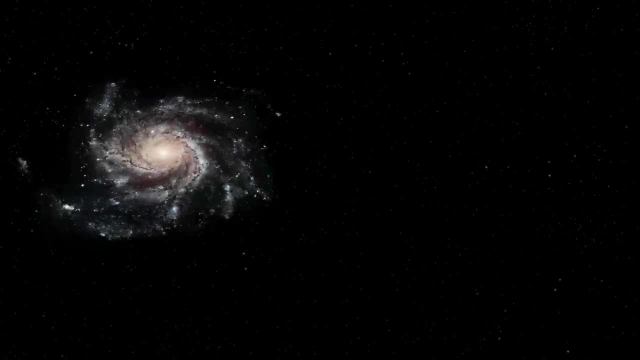 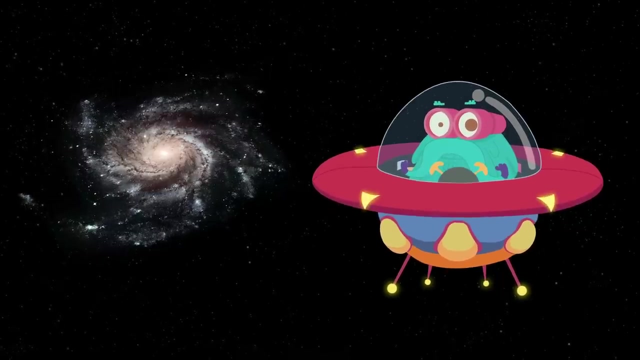 Does that make you raise your eyebrows? Time for me to get back to Earth. Tune in next time for more fun facts. This is me zooming out, Hey friends, wondering where I am right. Well, I am in space. 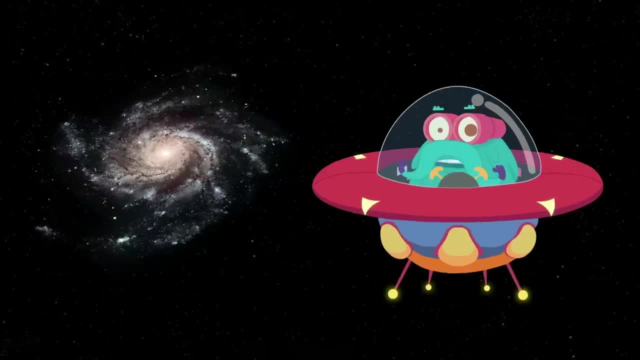 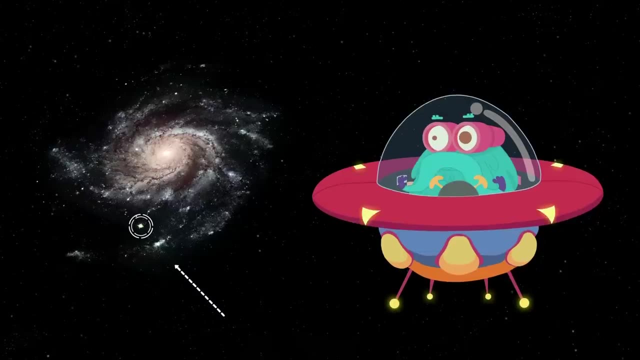 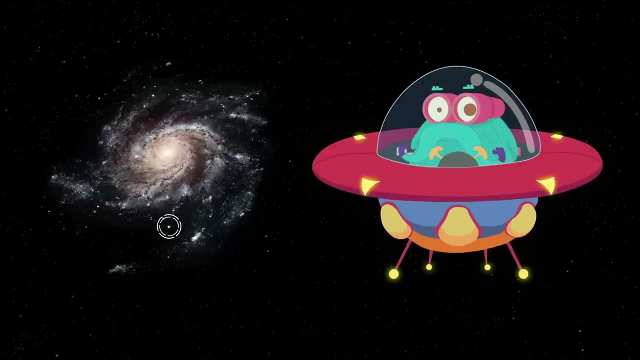 And do you know what that is? That is our galaxy and it's called the Milky Way. Do you see that? That bright light is our solar system? That's where we live. Come, let's take a closer look at our solar system. 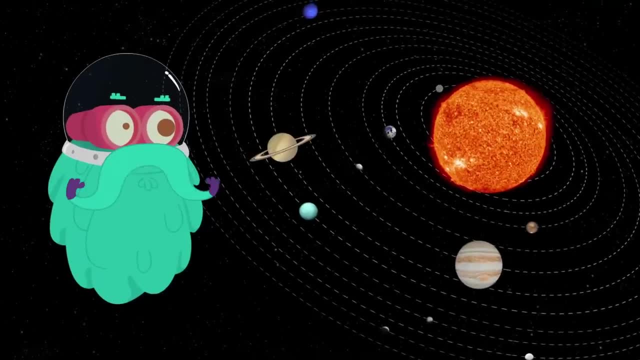 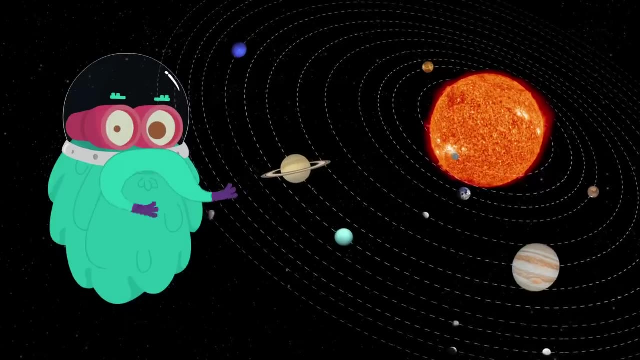 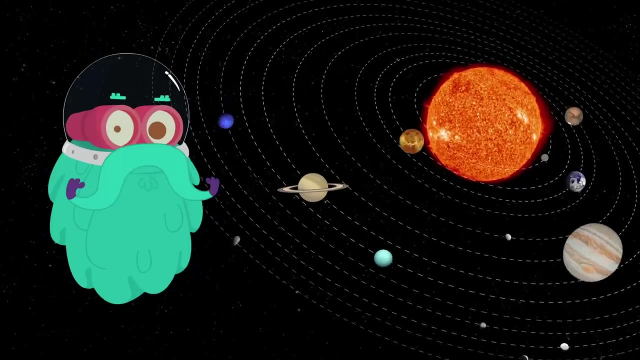 Zoom in. This is how our solar system looks like, with planets revolving around the sun. The sun is the main source of light for all the planets. Our solar system has 8 major planets: Mercury- Mercury is the closest planet to the sun. 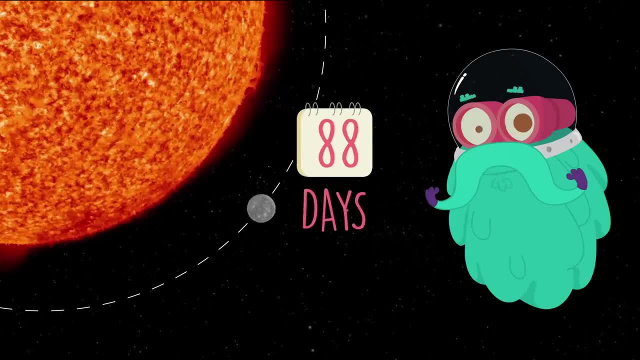 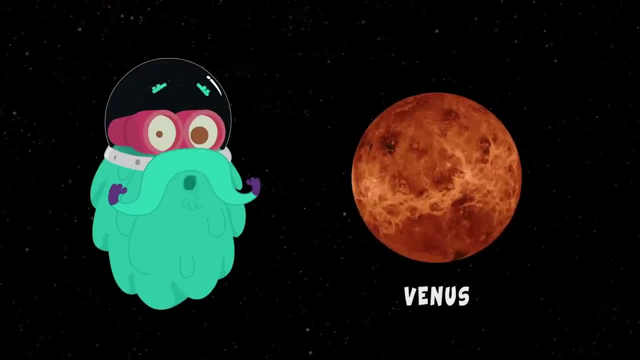 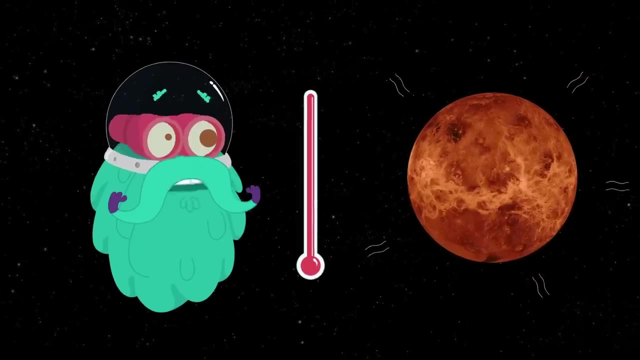 A year in Mercury is 88 days long And you know what You will see: Mercury from Earth in the year 2016.. Venus- Venus is the second planet from the sun And it is the hottest planet in the solar system. That's because it has high amount of carbon dioxide, which traps heat inside it. 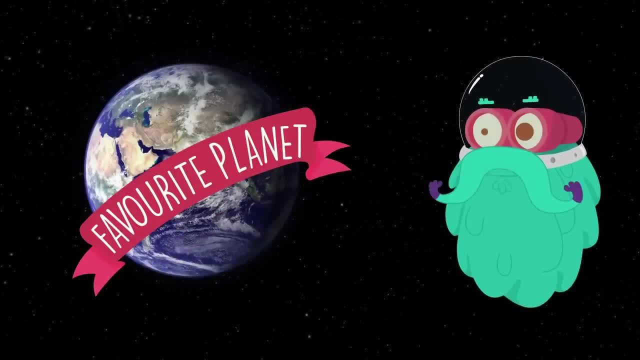 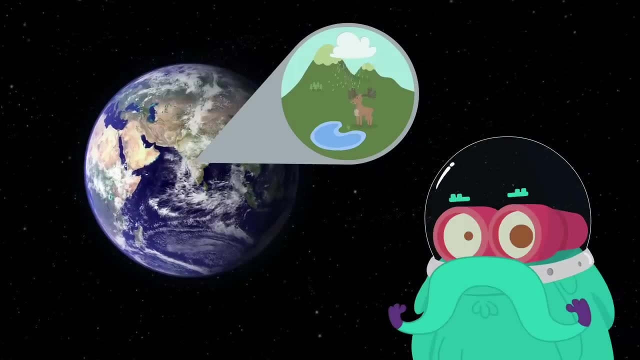 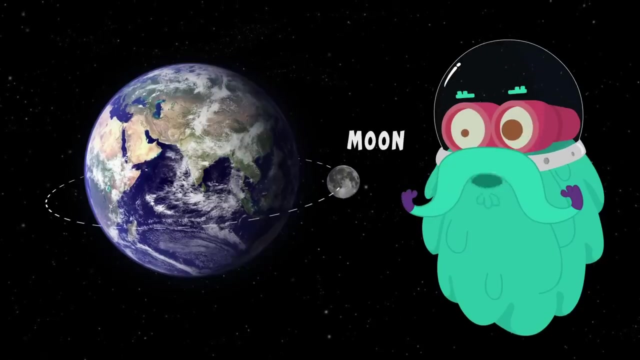 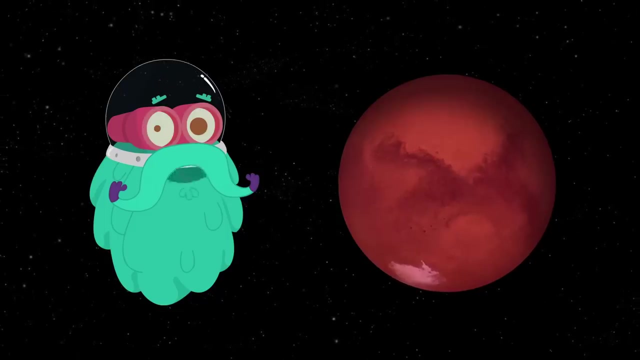 Earth. This is my favourite planet, for obvious reasons, of course. Earth is a unique planet with suitable climatic condition, landforms and water bodies Which support life in all forms. Moon is the natural satellite of Earth, Mars- Mars is often known as the red planet because of its reddish appearance. 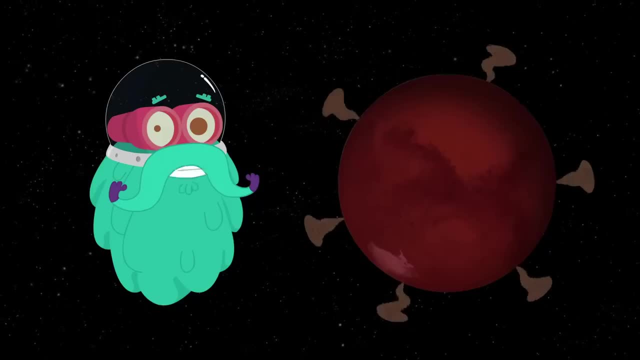 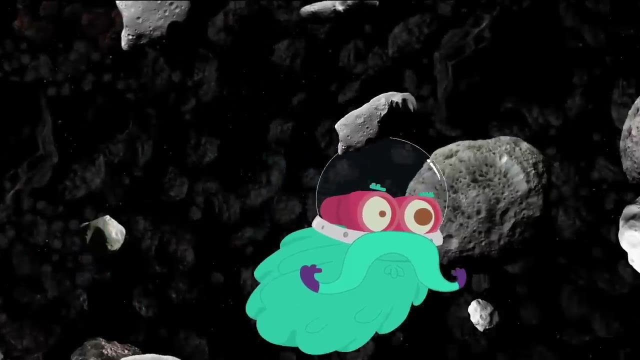 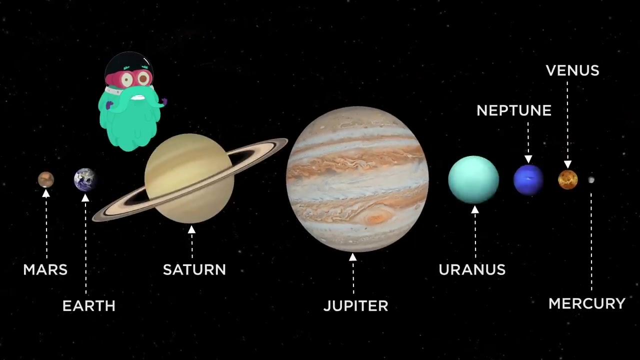 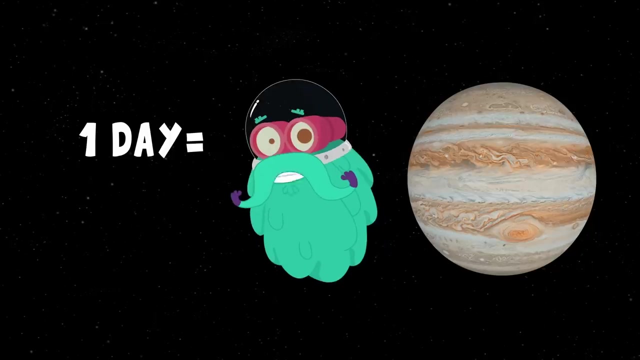 It is home to some of the largest dust storms, which can continue for months and cover the entire planet Jupiter. Jupiter is the largest planet of our solar system. It also has 4 moons. One day in Jupiter is just about 9 hours 55 minutes. 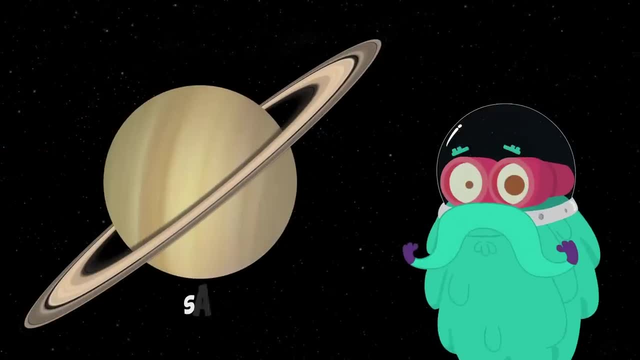 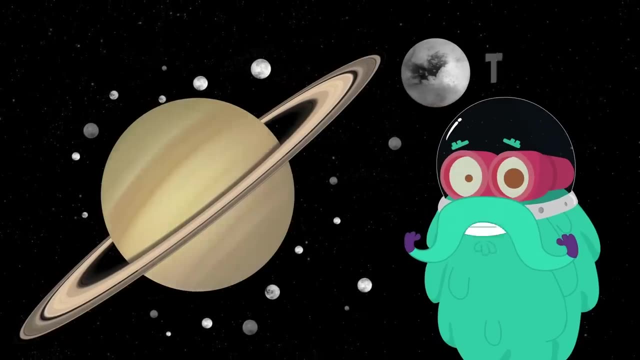 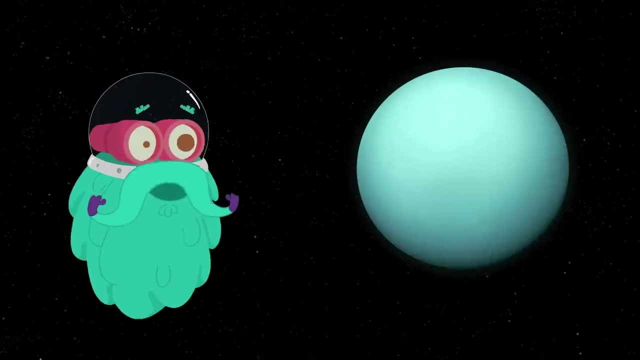 Making it the shortest day of all planets, Saturn. There are about 150 frozen moons around Saturn. The largest one is called Titan. This planet has beautiful rings around it made of dust and ice- Uranus- Uranus is a very, very cold planet. 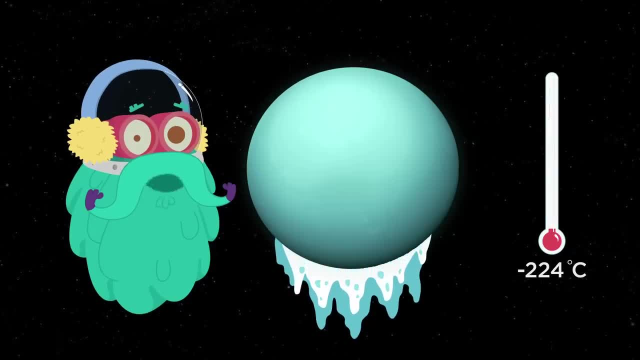 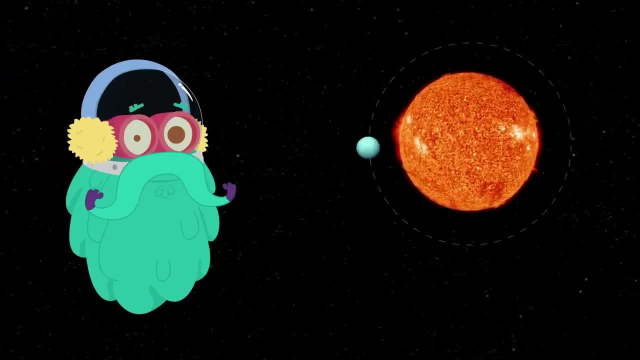 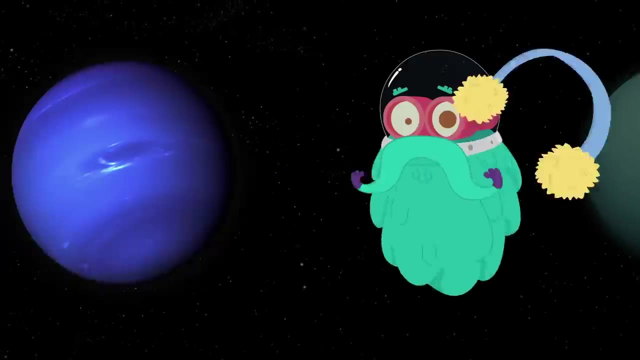 With temperatures dropping to about minus 224 degree Celsius. It takes about 84 earth years to revolve around the sun, Out of which it gets direct sunlight for 42 years And the rest remain in darkness. Neptune- Neptune- takes about 165 earth years to revolve around the sun. 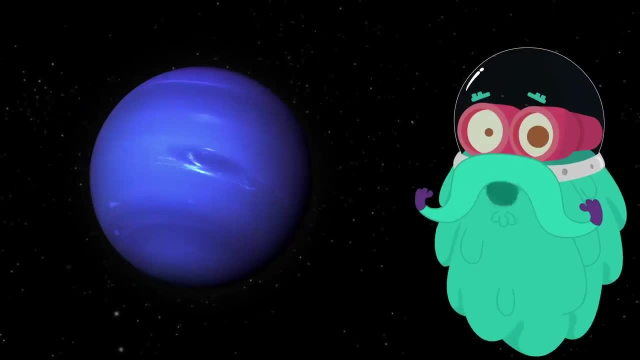 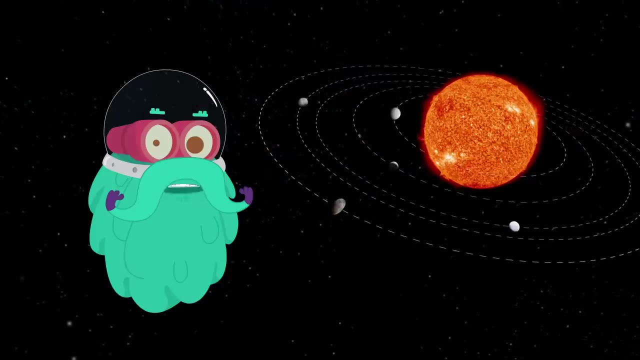 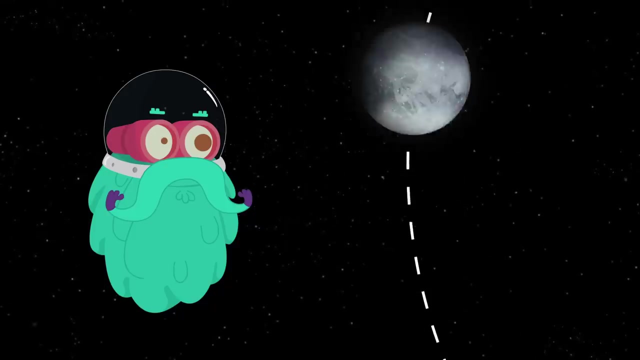 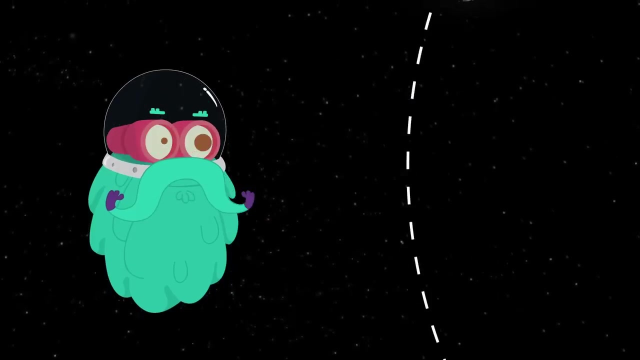 It is also known as the ice giant And it has about 14 moons Trivia time. Did you know that we also have 5 dwarf planets in our solar system: Ceres, Pluto, Eris, Makemake And Haumea? 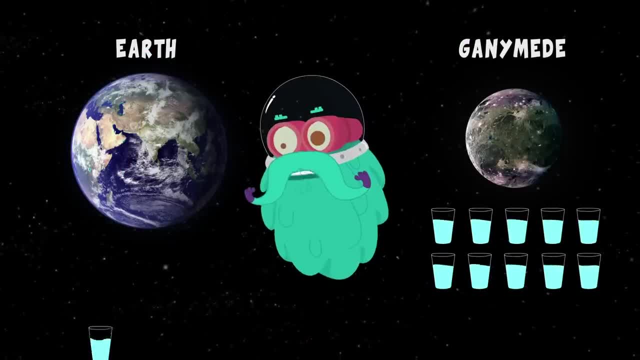 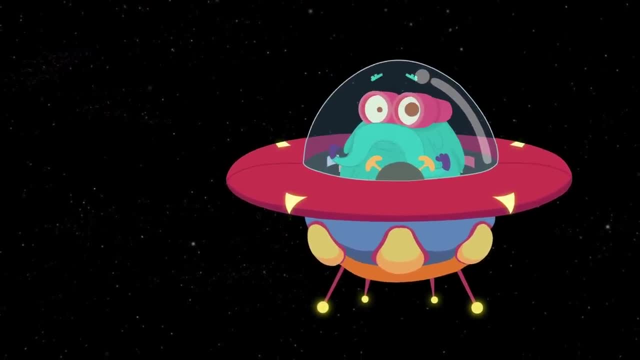 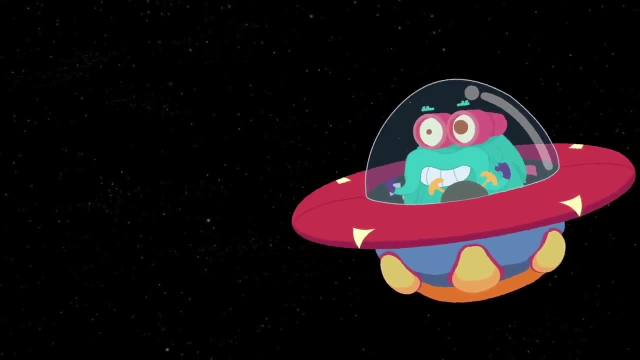 Jupiter's moon, Ganymede, has more water than the earth. Whoa, That's so much information for today. I am tired now, So this is me zooming out. Tune in next time for some more fun facts, Dr Binocs. 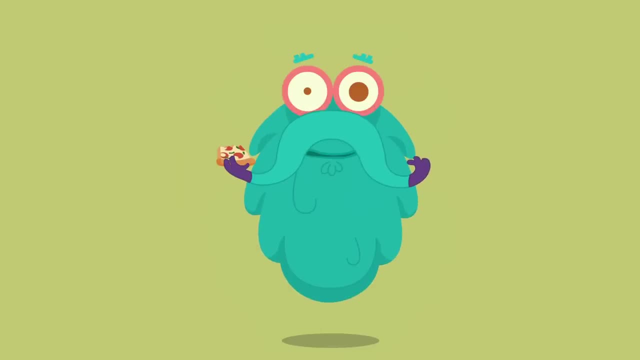 Dr Binocs. Oh hello friends, The best part of a pizza is its crust. Yummy. Just like this pizza, the earth too has a crust, But with no cheese in it. So let's learn something about the structure of the earth today. 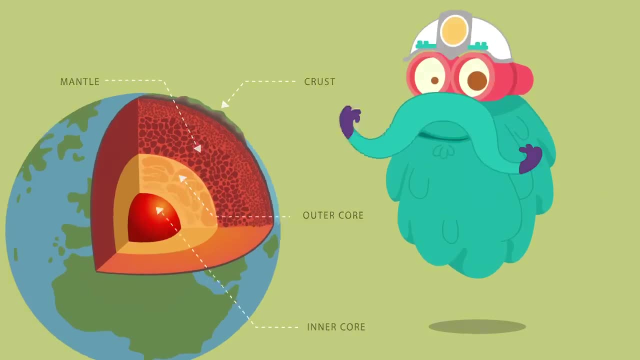 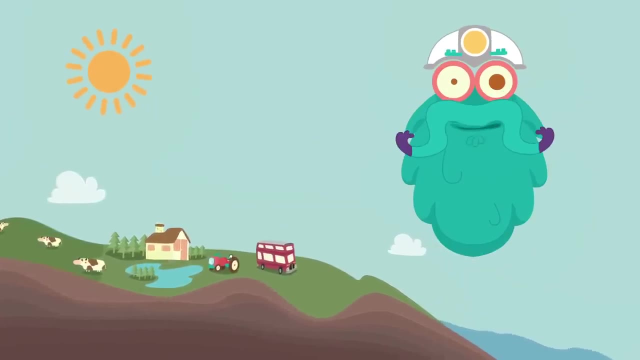 It consists of the crust, mantle and core. Zoom in. This is the earth's crust. It consists of all kinds of rocks, soil and everything you see above the earth's surface. You will be surprised to know that the crust, that is the land on which we walk, is almost 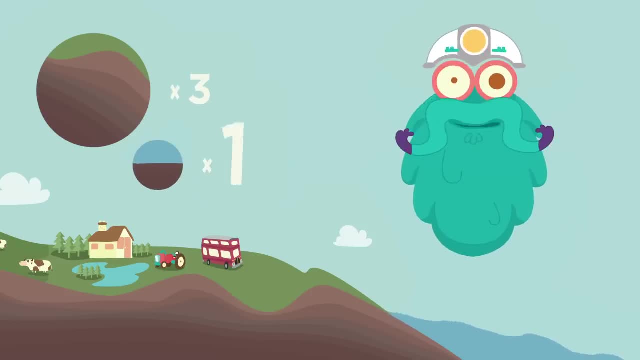 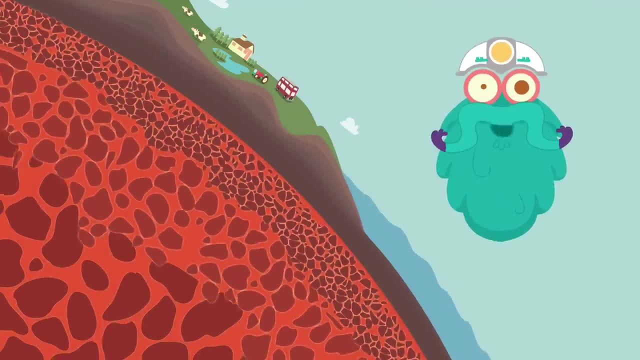 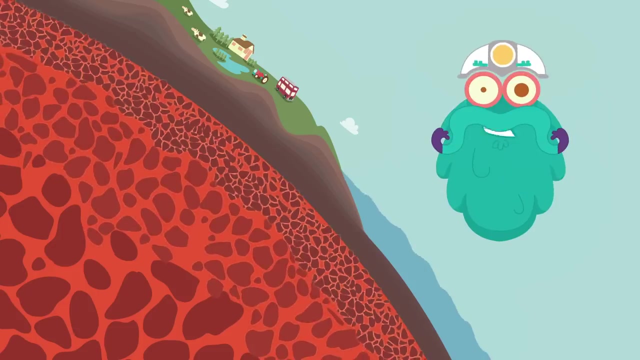 3 times thicker than the crust under the oceans And it extends to about 25 miles. The earth's crust floats on this layer, which is called the mantle. It is made of thick, solid rocky substance and amounts to about 85% of the total mass of earth. 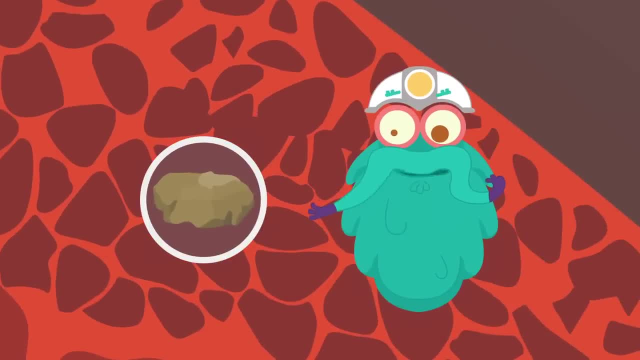 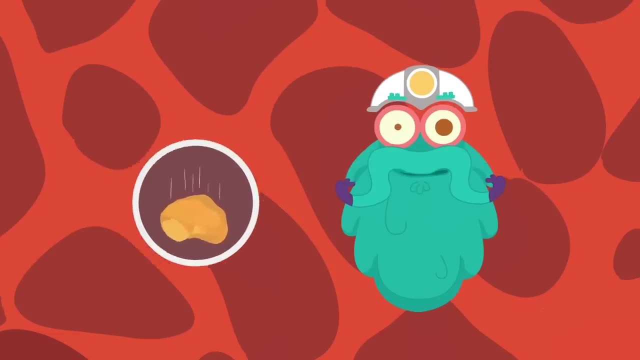 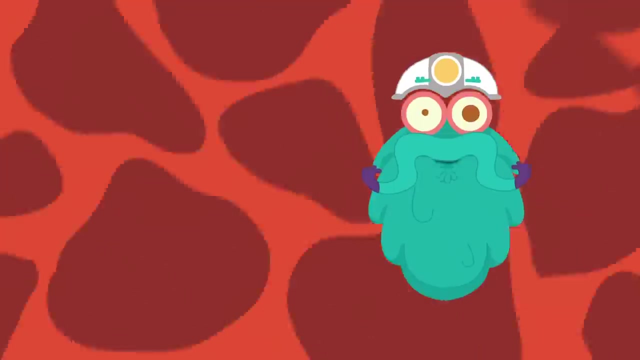 The first 50 miles of the mantle consists of very hard, rigid rocks. The next 150 miles are made up of super hot, solid rocks. Below that, for the next several hundred miles, the earth's mantle is believed to be made up of very solid and sturdy rock materials. 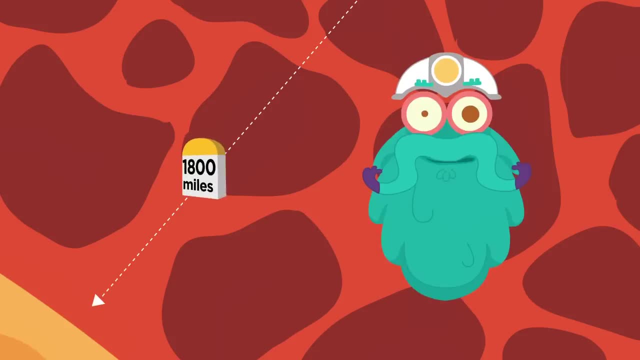 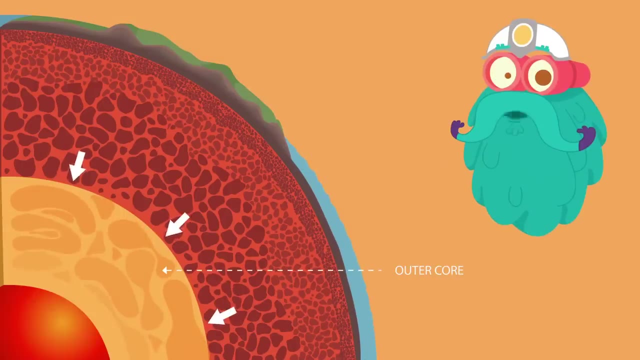 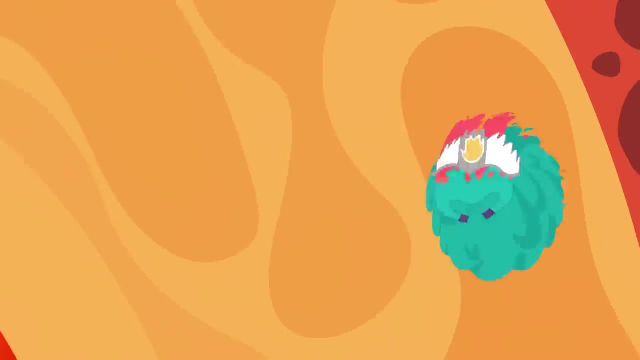 The mantle is about 1800 miles thick and by far the largest layer of earth. The earth's outer core is made up of super hot liquid, molten substance called lava. This lava is believed to be made of iron and nickel. It extends to a depth of 3000 miles beneath the earth's surface. 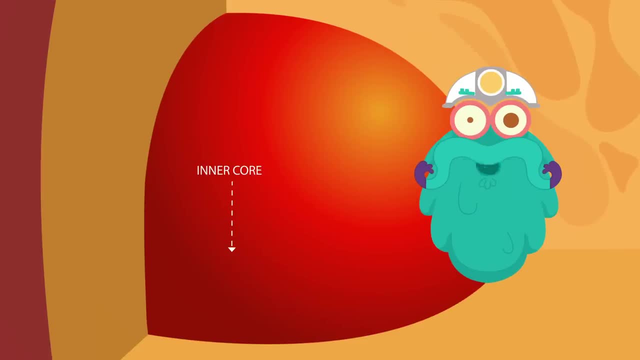 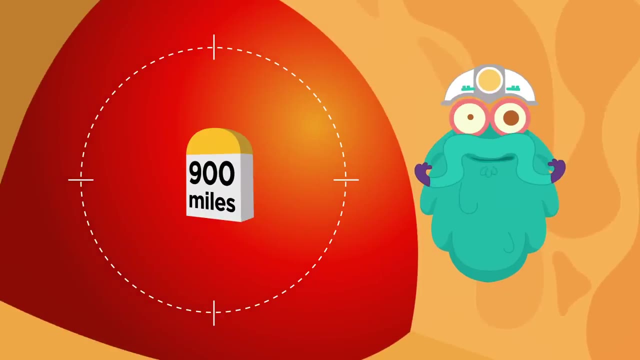 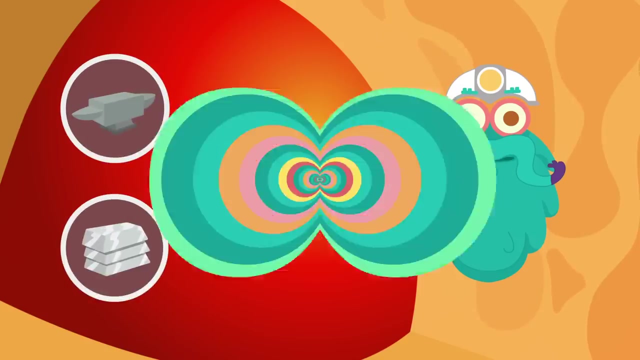 And finally we have reached earth's inner core. The inner core extends another 900 miles towards the center of the earth. It is believed that this inner core is a solid ball made of iron and nickel- Trivia time. The crust occupies less than 1% of earth's volume. 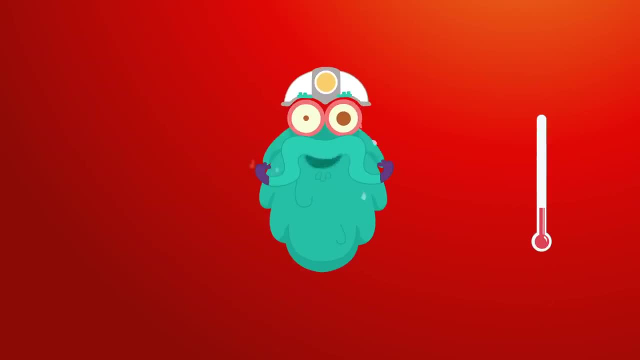 The inner core is the hottest part of the earth, and it is as hot as the surface of the sun. Surprising, isn't? it Looks like it's time for me to zoom out before I get baked in this heat. Tune in next time for more fun facts. 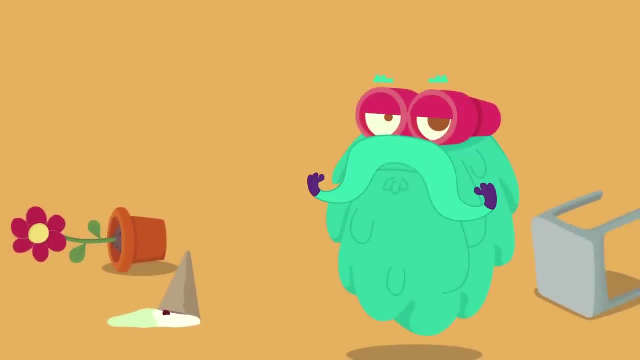 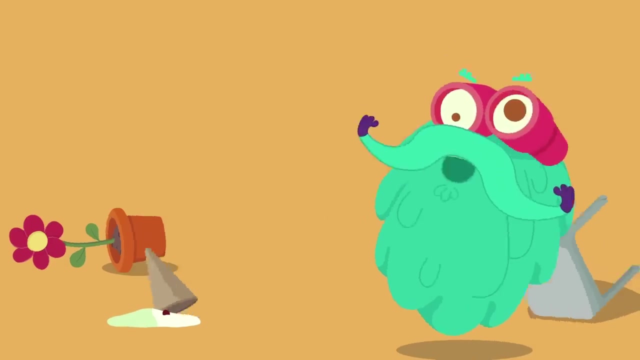 Whoa, You are laughing right Watching me tumble like that, Are you? Oh no, no, Go ahead. But hey, do you know what just happened? There? we go again. Well, this is nothing but an earthquake. 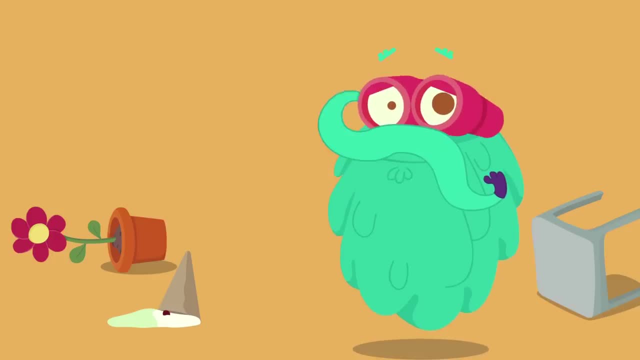 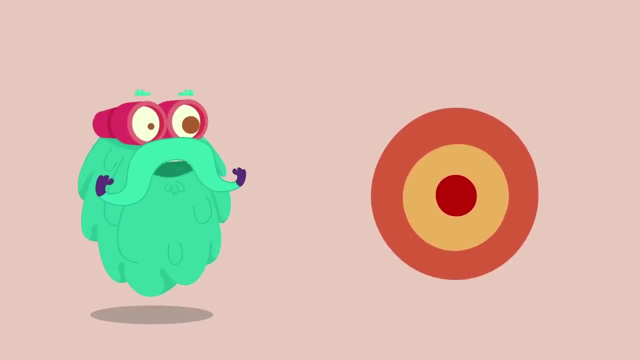 A small one indeed. Come let me tell you about earthquakes today. Zoom in: The surface of the earth is like a jigsaw puzzle. Yes, it's not a single piece of land, But it's like a jigsaw puzzle. The earth's surface is like a jigsaw puzzle. 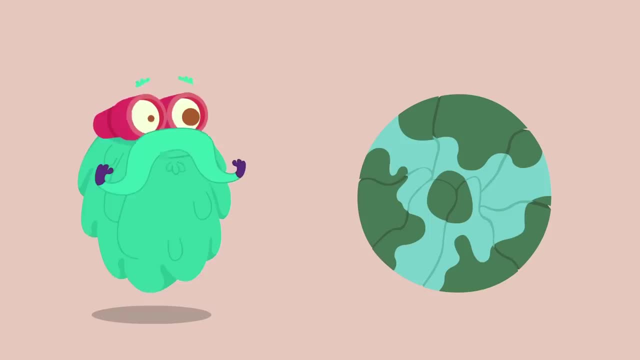 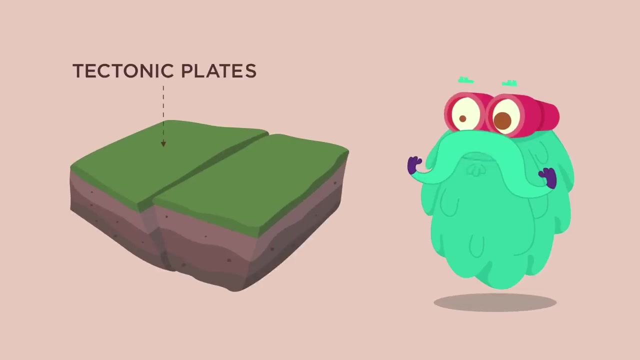 Yes, it's not a single piece of land, but approximately 20 pieces of a puzzle that constantly move, But you don't feel it because they move quite slowly. Each one of those puzzle pieces are called tectonic plates, So whenever those plates hit, bump or slide past another plate, an earthquake is caused. 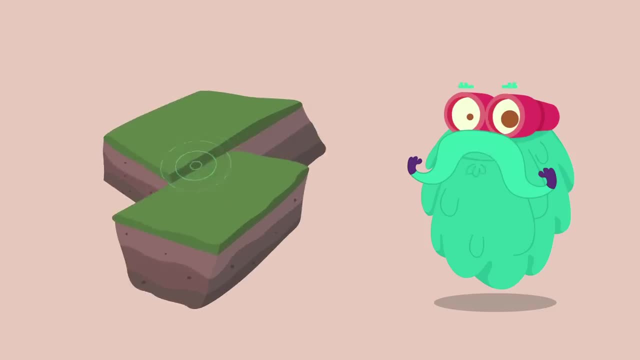 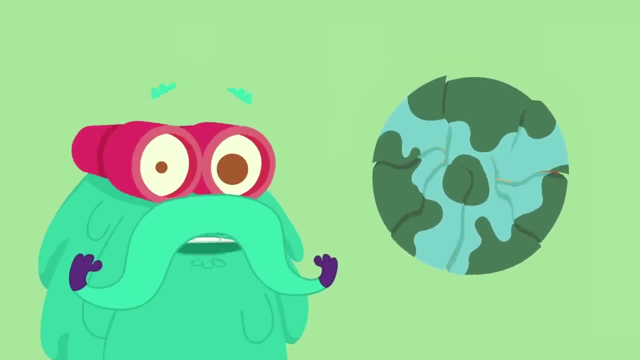 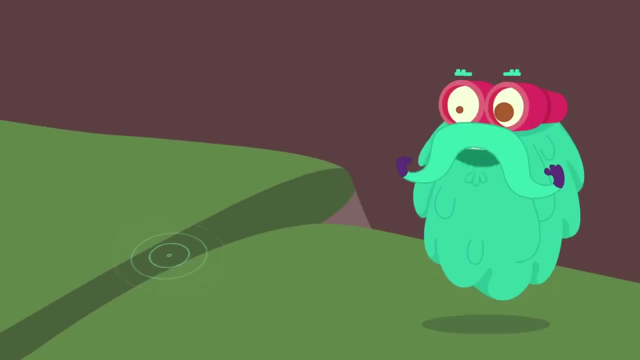 The surface where these plates slip is called the fault or the fault plane. So when do you think it happens? Well, it happens all the time, But hey, don't be scared. Most of the times we don't feel the quakes, as they are too small to reach us. 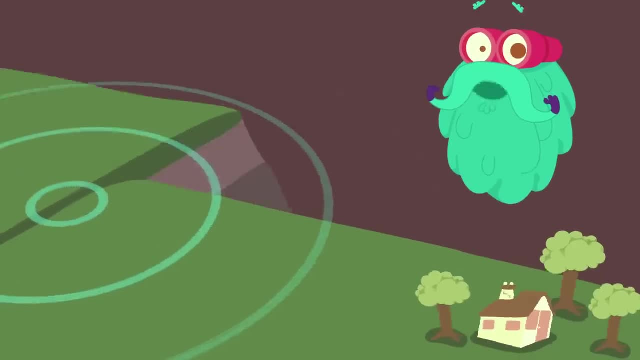 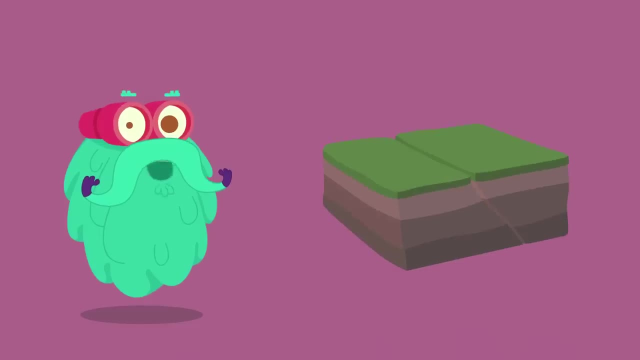 But sometimes they are so strong that they can be felt over a thousand miles away. The place where the earthquake originates is called the hypocenter, And the place where it occurs on the earth's surface is called the epicenter. There are three types of earthquakes. 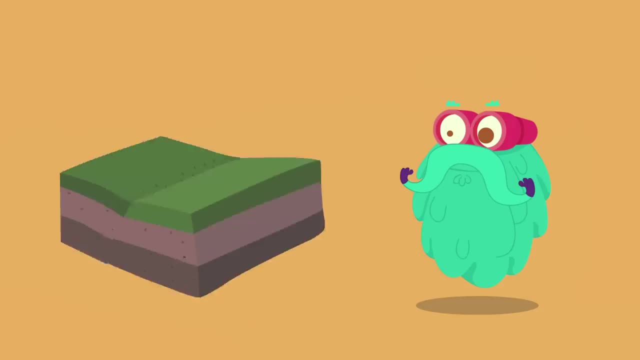 Convergent boundary: Here one plate is forced over another during an earthquake, which causes a thrust fault. Many hills and mountains have been formed due to the convergent boundary. Divergent boundary: Here plates are drifted apart from each other, forming a rift zone. 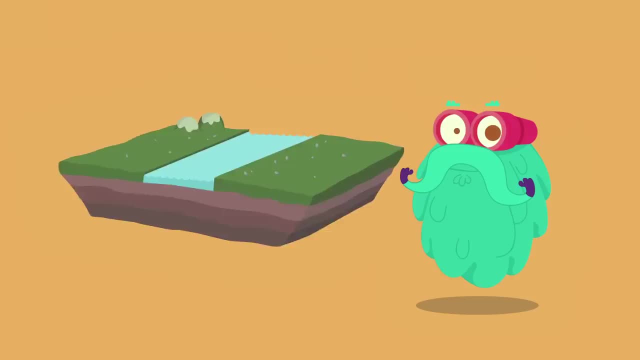 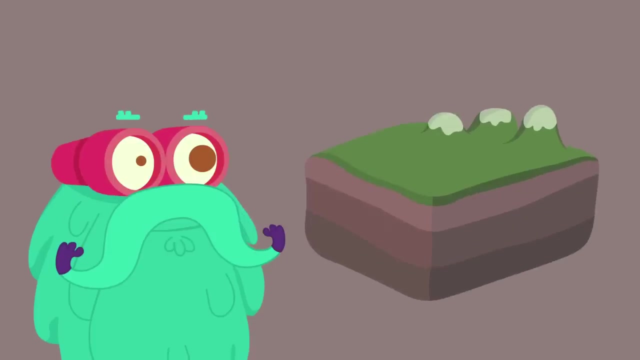 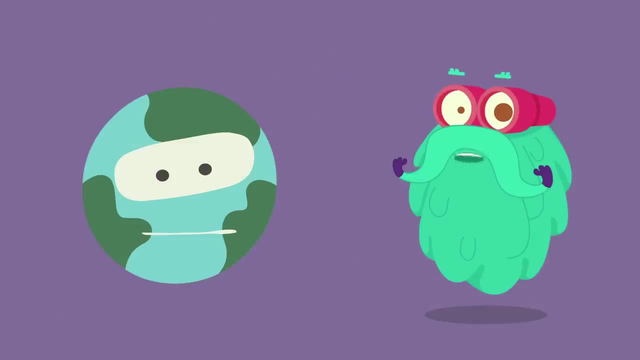 This kind gives birth to new ocean flows, Transform fault. Here the plates slip by each other And this is also called strike slip. So earthquakes are nothing but the shaking, Rolling Or a sudden shock of the earth's surface. Now you know that whenever the earth is stressed or angry, it shakes and grumbles. 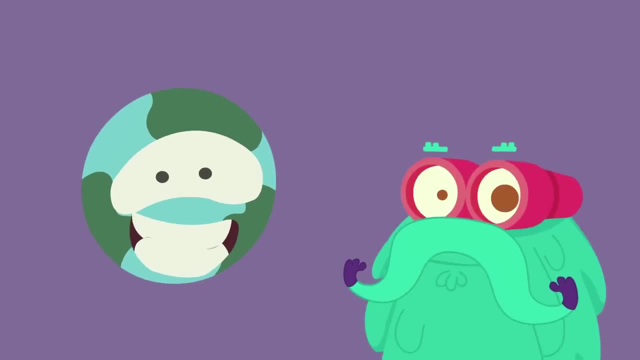 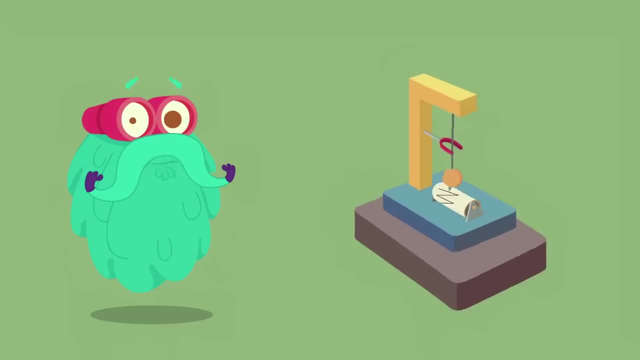 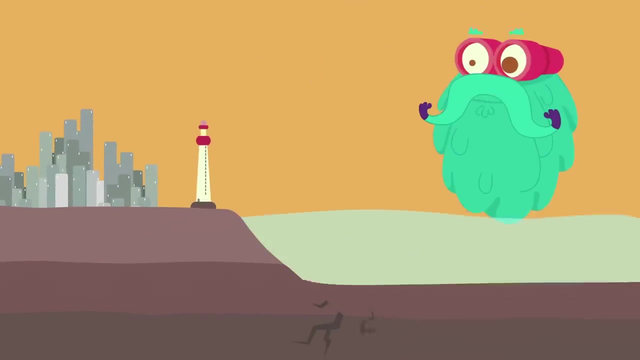 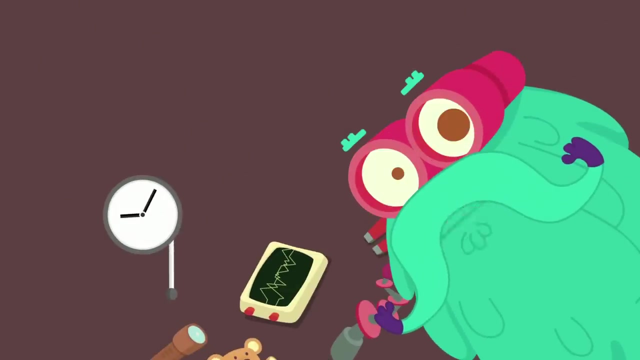 Don't be scared, I was just kidding, Trivia time. The instrument used by scientists to measure the intensity of earthquake is known as a seismograph. A tsunami is caused when earthquakes occur under water. Whoa Yikes. I need to rush before I tumble again. 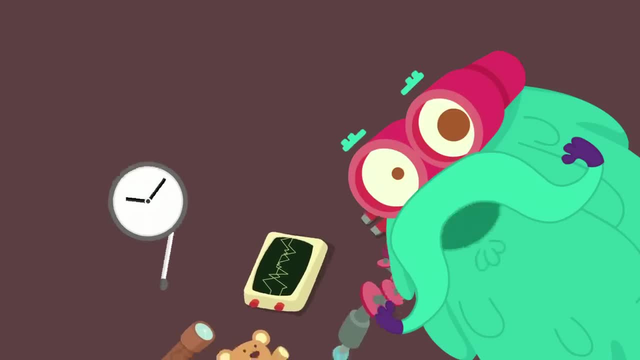 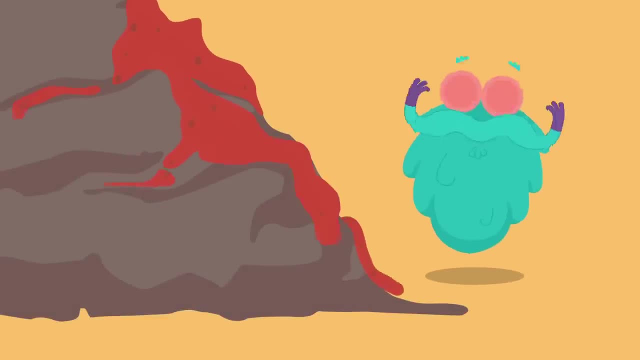 So this is me zooming out. Tune in next time for more fun facts. Oh, Hello friends, Are you wondering what this is? Well, it's the molten lava that comes out from a volcano. Come, let me tell you what a volcano is. 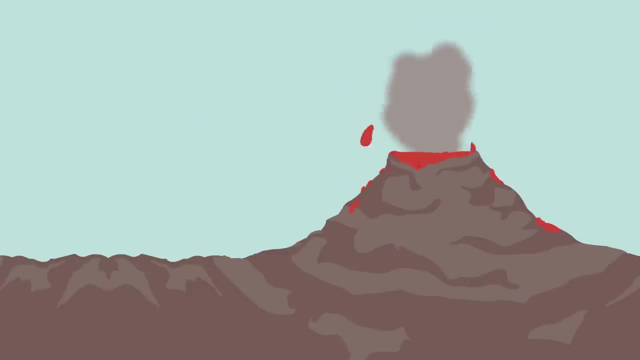 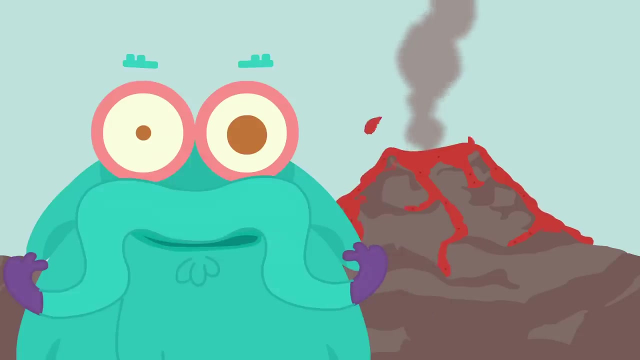 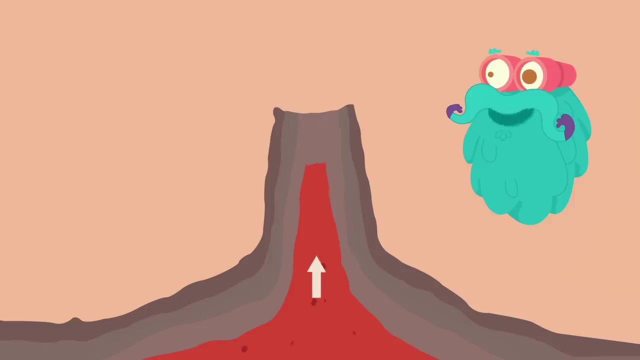 Zoom in. I'm sure you've seen mountains that open up and blurt out thick, molten, semi-solid like substance. Well, that's called a volcano. Let's learn more about it. A volcano is a vent or chimney that connects magma from within the earth's crust to the earth's surface. 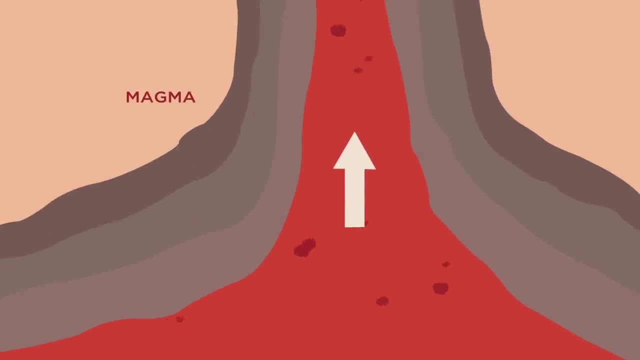 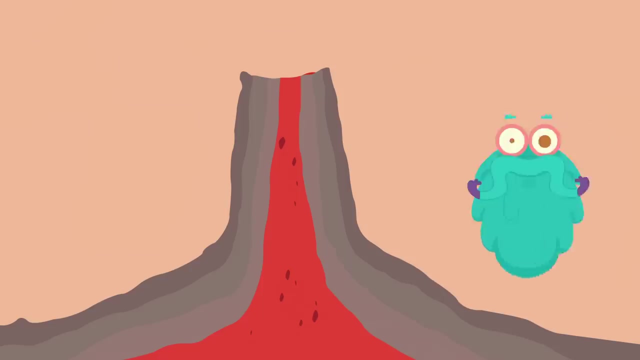 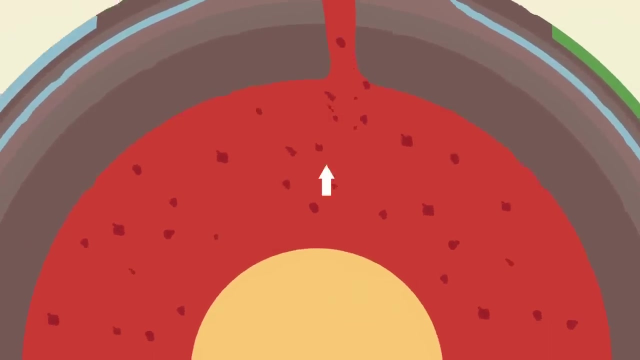 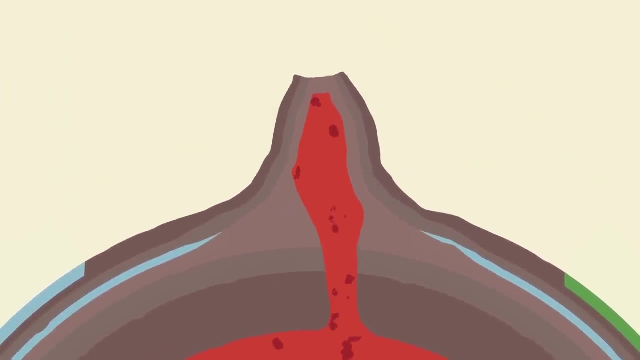 The liquid rock is called magma when it is under the earth's surface and lava after it comes out. So how does a volcano erupt? The molten rock stored in the magma chamber rises through the crater pipe pockets. As it travels up, the main vent gases expand and water becomes steam, creating pressure. 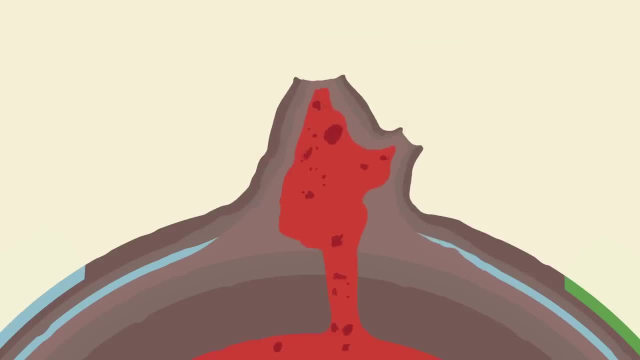 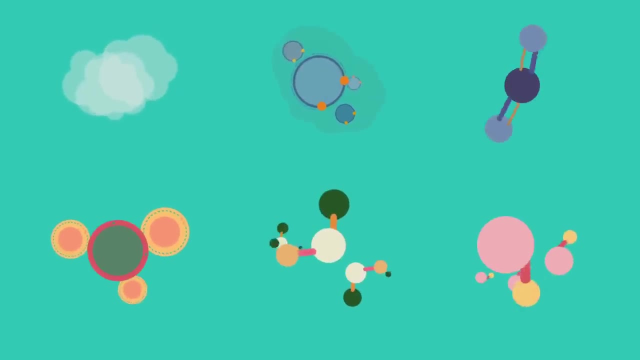 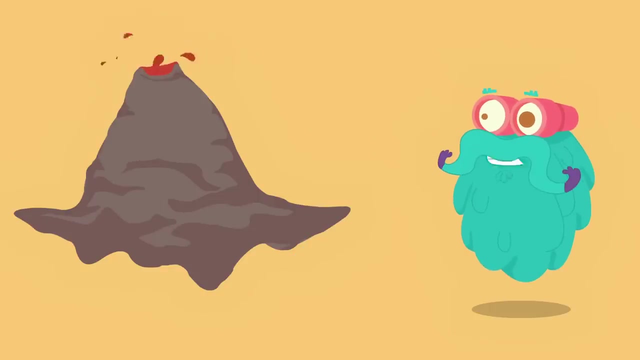 When the pressure can no longer be contained, the volcano erupts through the crater and secondary side vents. Common volcanic gases include water vapor, carbon dioxide, sulfur dioxide, Hydrogen chloride, hydrogen fluoride and hydrogen sulfide. Popular belief is that volcanoes are large, cone-shaped mountains, but that's not true. 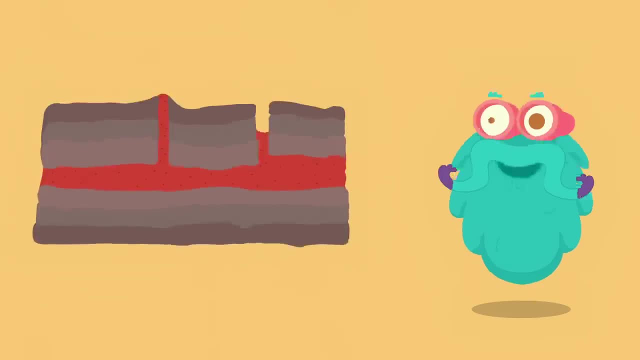 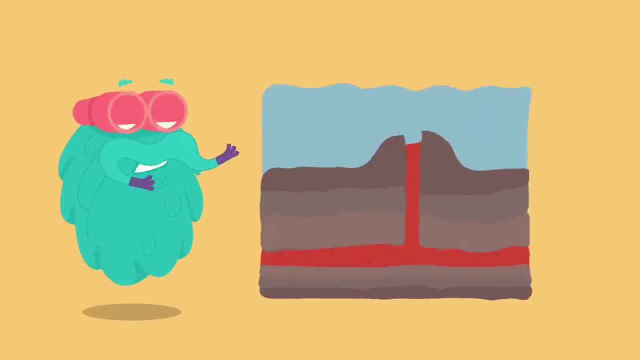 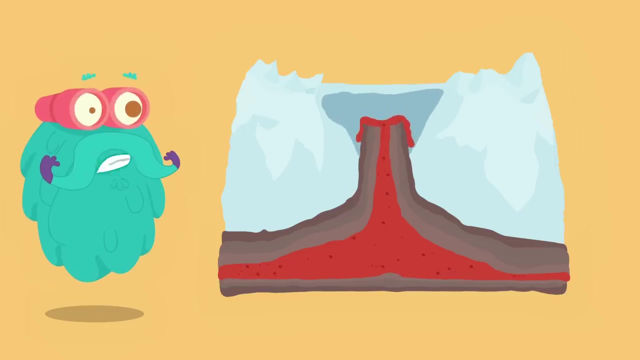 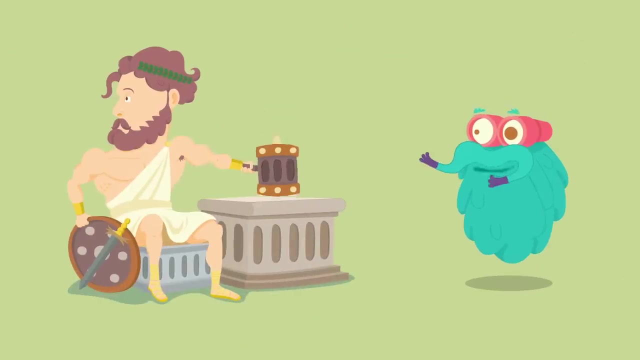 There are many more types of volcanoes, such as white plateaus, fissure vents and bulging dome shapes. There are also volcanoes found on the ocean floor and even under ice caps, Such as those found in Iceland. The word volcano originally comes from the name of the Roman god of fire, Vulcan. 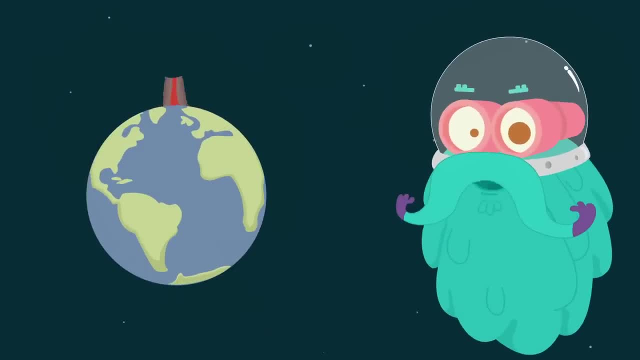 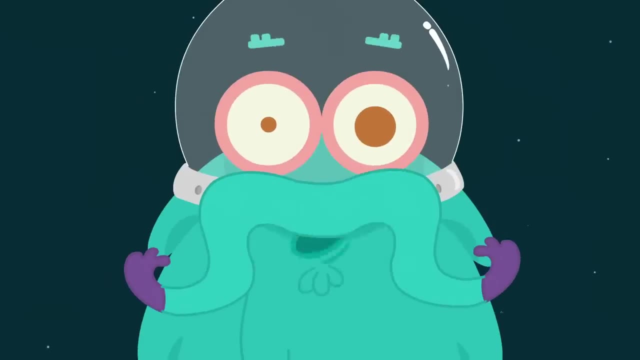 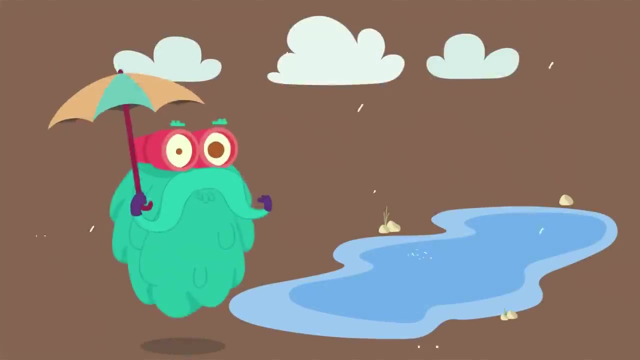 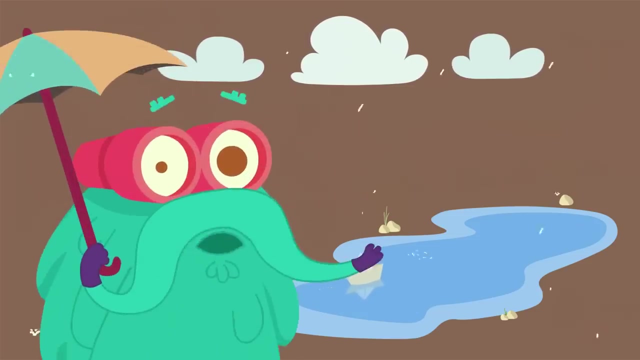 The tallest volcano in the solar system isn't on earth at all, but on Mars. So tune in next time for some more fun-filled facts. This is me zooming out. Ah, It's raining. Hey, Have you ever wondered where the rain comes from? 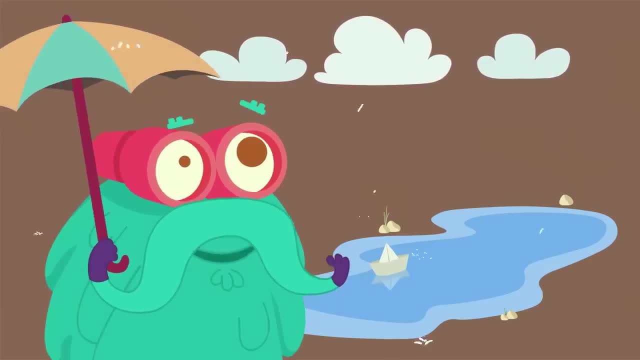 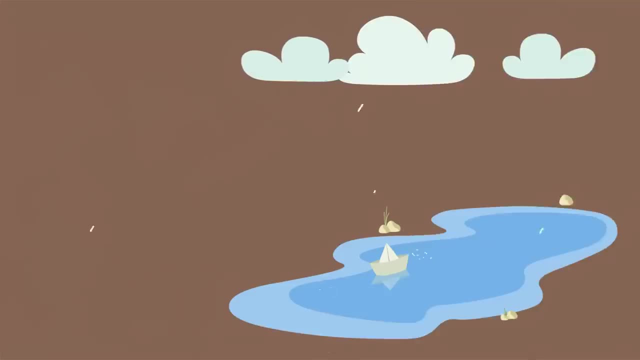 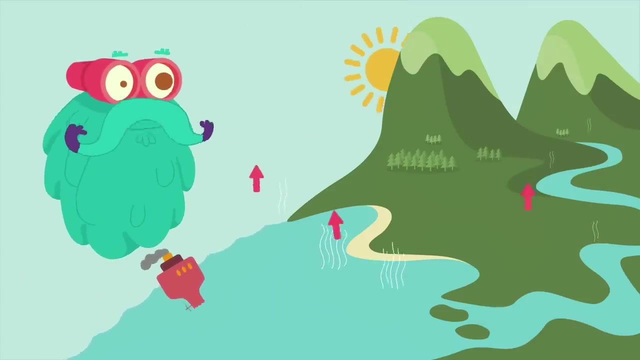 Or how the clouds are formed. Well, this is what the water cycle is all about. Come let's explore. Zoom in. When the sun heats up the rivers and oceans, water becomes water vapor And it rises up in the air. 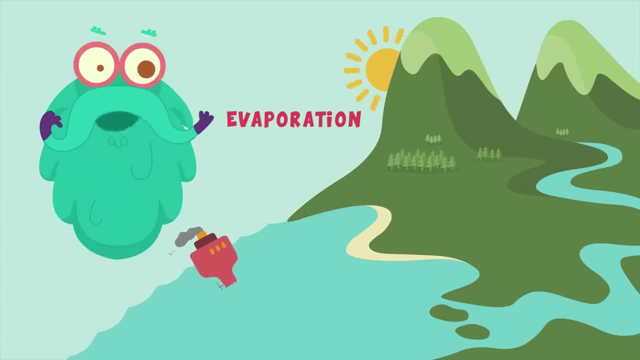 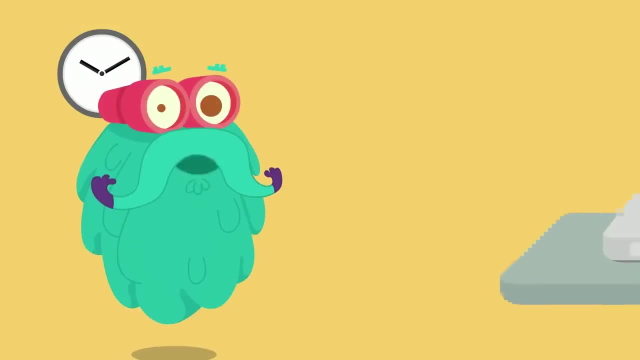 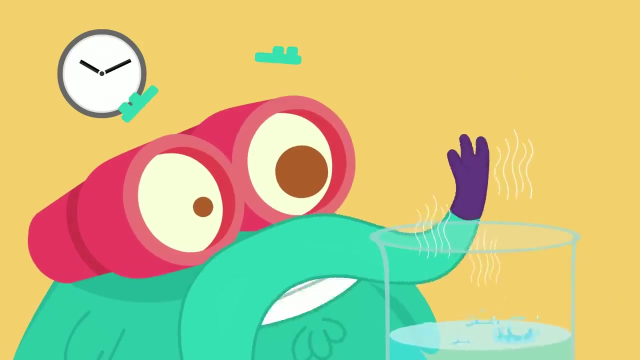 This process is called evaporation. It is the first step of the water cycle. You too can see water vapor at home. Just tell your mummy to heat some water, And as the water gets heated, you'll be able to see the water vapor rising up in the air. 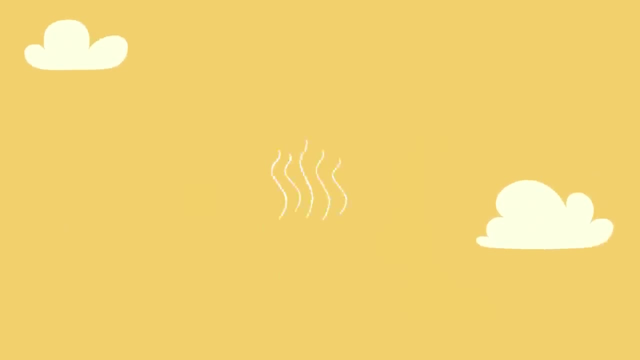 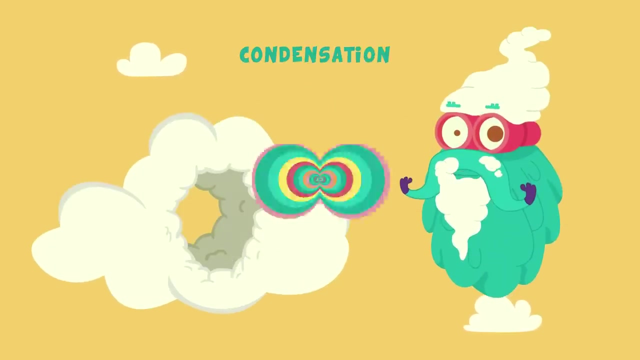 When the water vapor reaches up in the sky, it turns into tiny droplets of water. These water droplets, along with various gases and dust particles, come together to form clouds. This is known as condensation. Now hold a cold lid over the vessel in which you heated water. 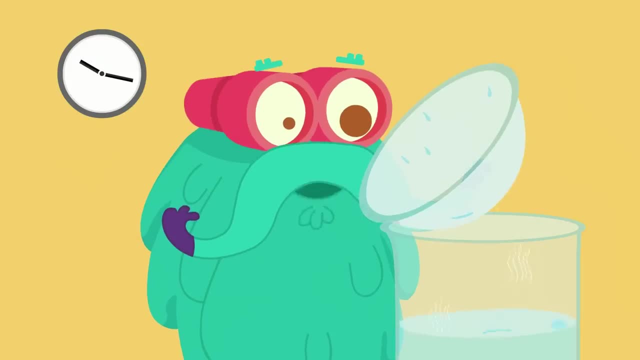 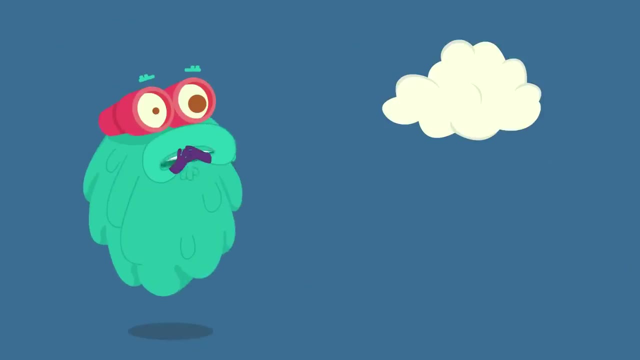 When you open the lid. after some time you'll be able to see water droplets on the lid. That's exactly what condensation is. When the cloud becomes too heavy and it cannot hold any more water inside, it bursts open to give out rain, hail or snow. 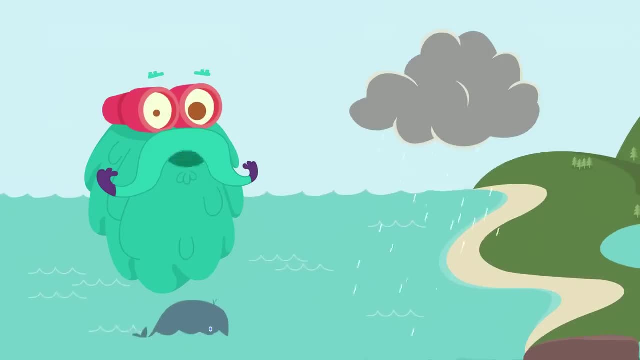 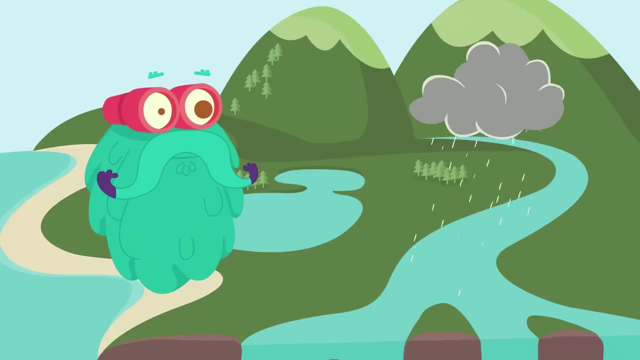 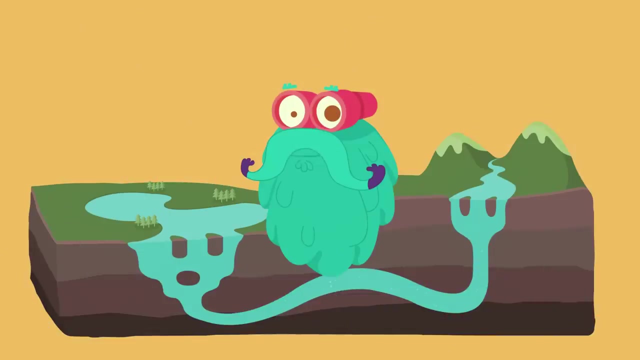 This is known as precipitation. As it rains, water gets collected in oceans, lakes and rivers. It even seeps through the soil and becomes groundwater. Thus, water cycle is a continuous process of evaporation, condensation and precipitation. Trivia Time: 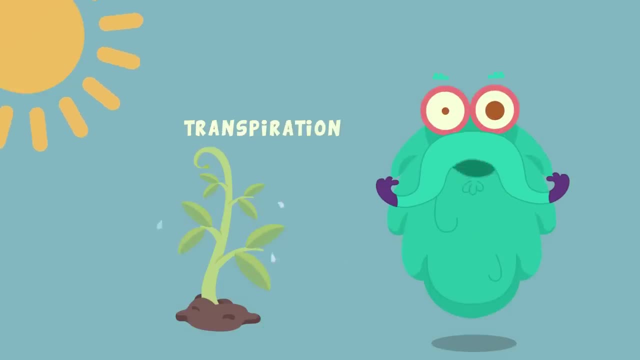 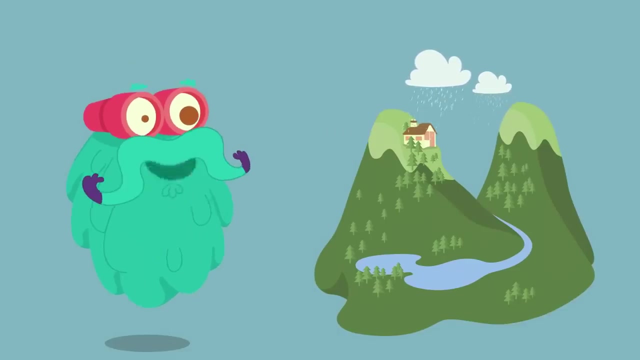 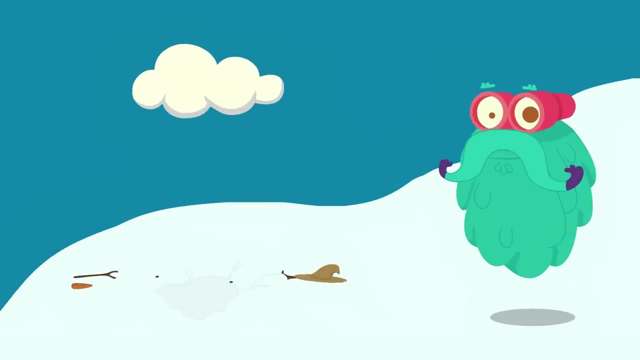 Did you know that even plants sweat? That's called transpiration. That's why it rains more in places with more trees, like hill stations and forests. Sometimes snow directly turns into water vapor without melting into water. That's called sublimation. 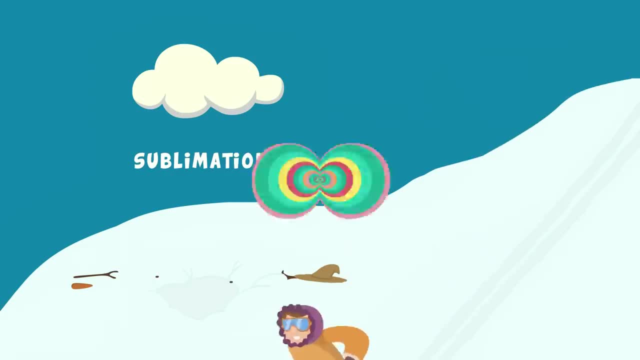 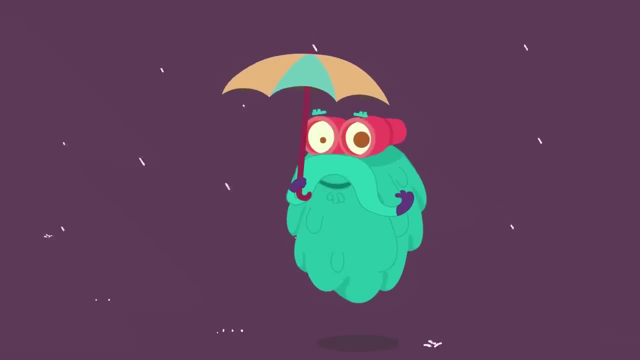 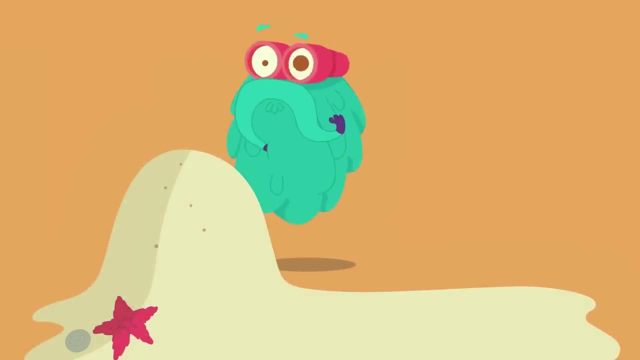 This happens a lot in cold countries. Oh, I need to run. now It's raining again, So this is me zooming out. Tune in next time for some more fun facts. Did you see that? Look how the water flows from the top of this mini hill and gets collected here? 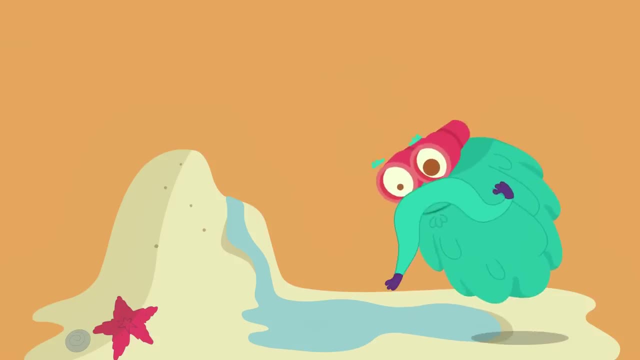 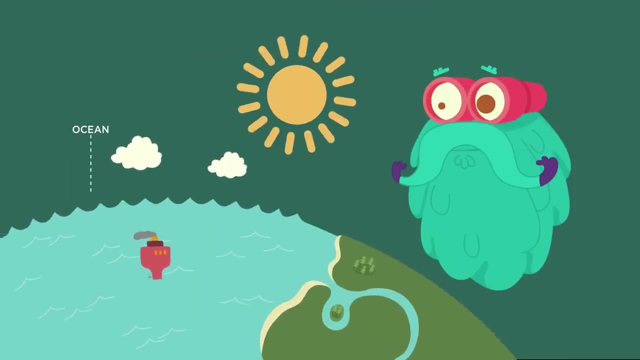 This looks like a river and this looks like a lake. Are you getting confused? Don't be Come. I'll tell you more about the water bodies on earth. Zoom in Ocean. Oceans cover more than 70% of the earth's surface. 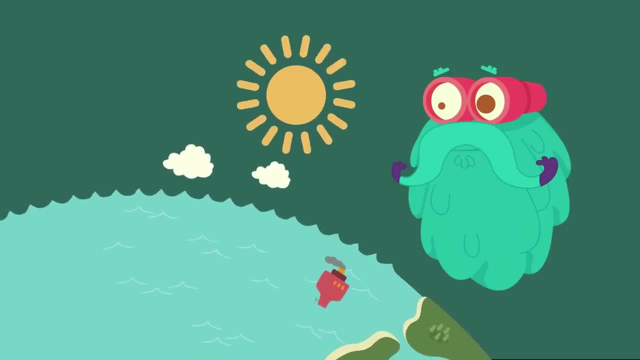 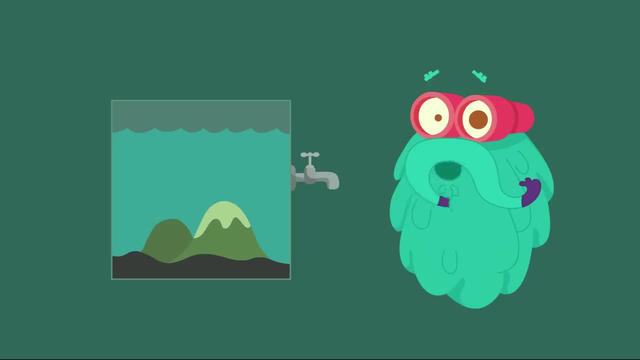 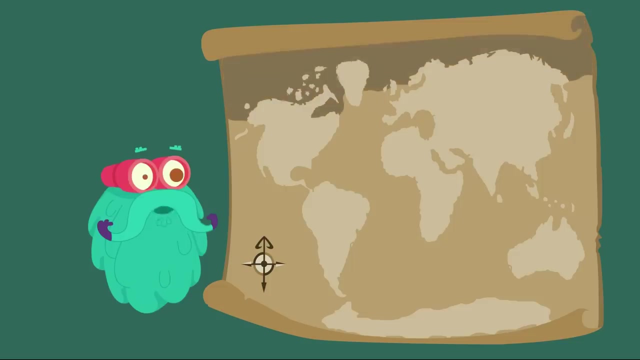 But that's too much water, isn't it? Then why do we have water problems all around? Yuck Well, because ocean water is salty and not safe to drink. The oceans of the world are the Arctic, Atlantic, Pacific, Indian and the Antarctic Ocean. 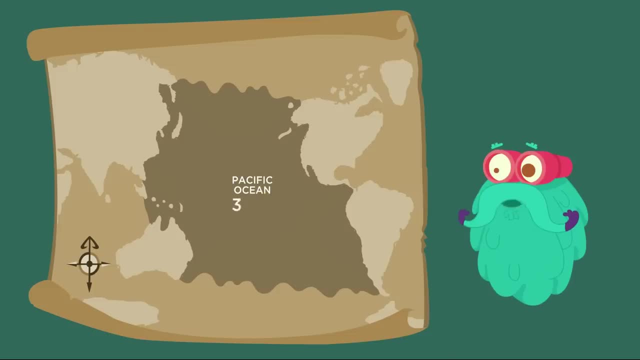 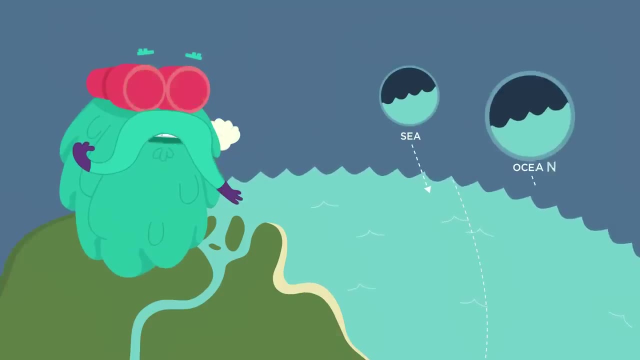 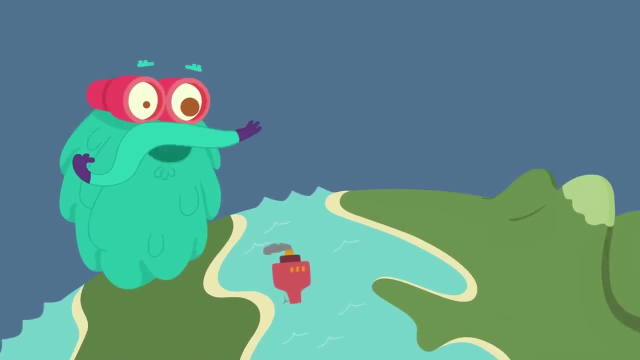 The Pacific Ocean is the largest and covers around 30% of the earth's surface Sea. The sea is found where the land meets the ocean. It is smaller than the ocean and is actually a part of it, Just like how the Mediterranean Sea is a part of the Atlantic Ocean. 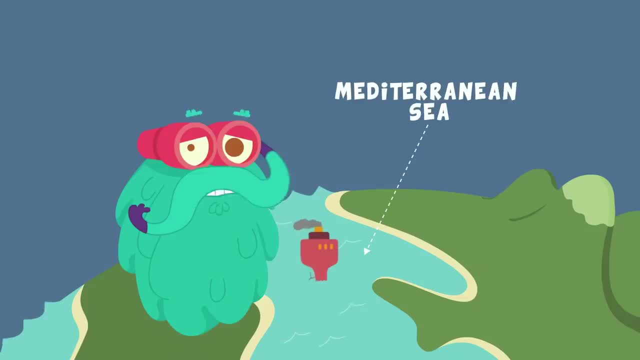 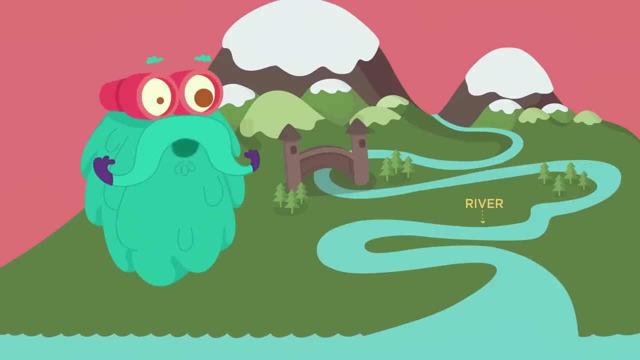 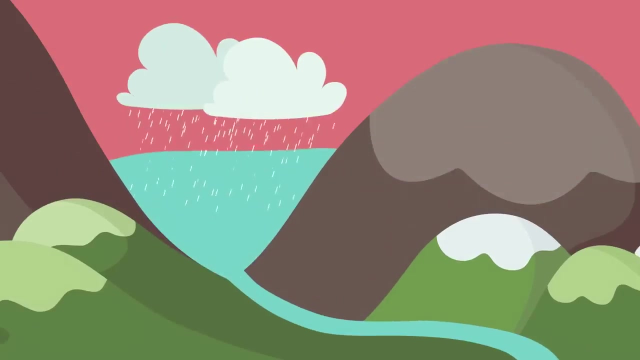 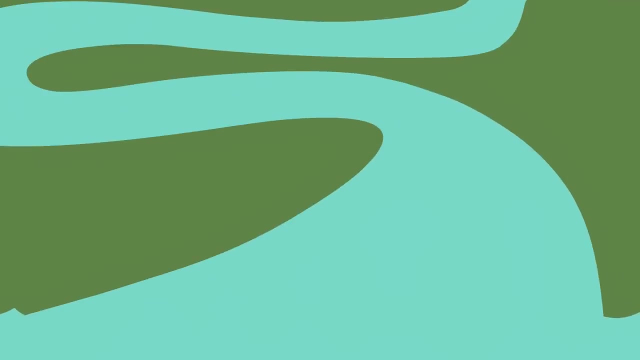 It also has the most confusing spelling River. A river is a strip of water that flows through many places. It begins in mountains or hills where melted snow and rainwater gets collected. The beginning of a river is called the source and the end is known as the mouth. 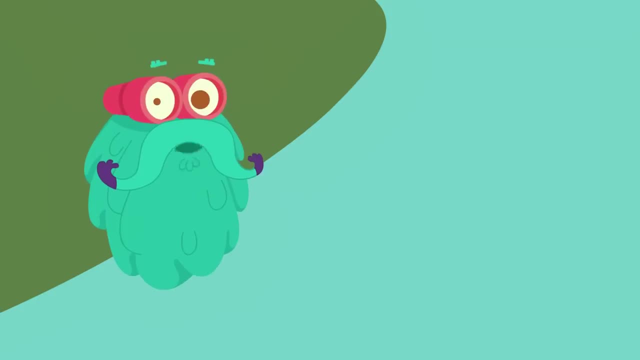 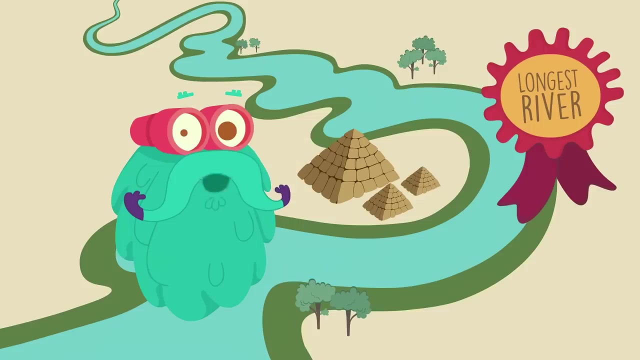 And there's some good news for you. Rivers contain fresh water. Well, by fresh water, I mean water that is suitable for you to drink. River Nile is the world's longest river, which passes through seven countries, Egypt being one of them. Lake 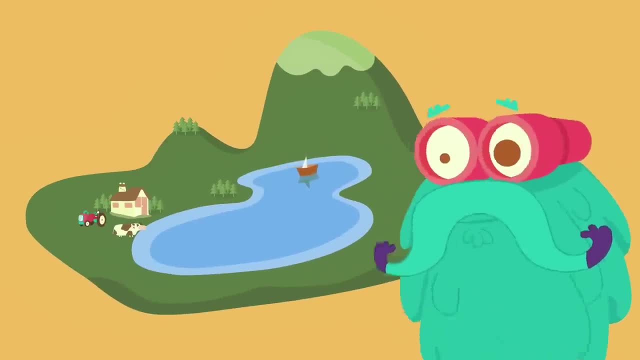 A lake is a large area of water surrounded by land. Lakes are formed when water finds its way into a basin. It could be through rain or underground water. It will be quite sad for you to know that lakes need a continuous source of new water. 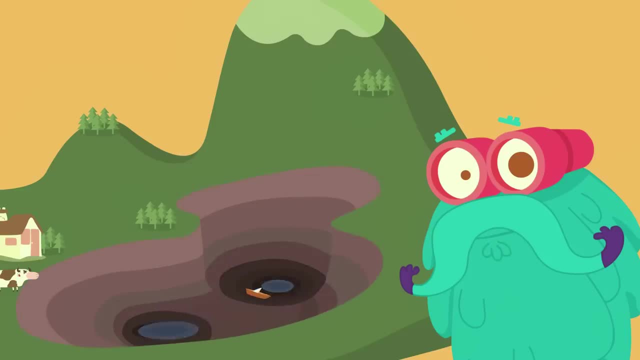 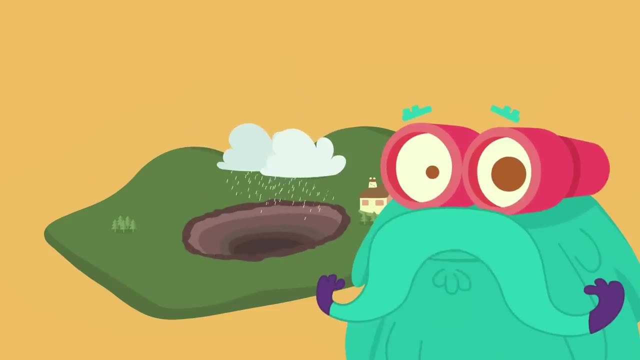 Otherwise they tend to dry up. Whoa, There you go. Sometimes lakes are formed when meteors hit the earth, So it's not always bad when a big, bulging meteor crashes on the earth's surface. Trivia Time. 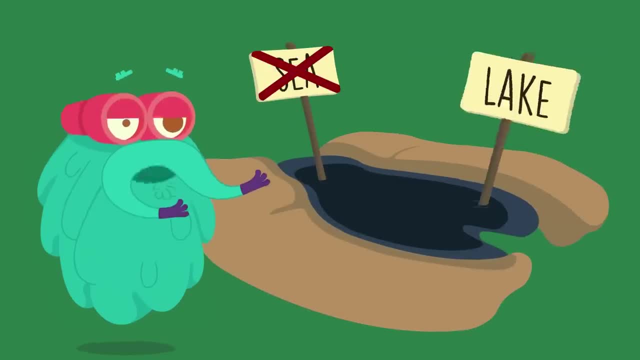 The Dead Sea is not a sea, but a lake. The reason why it's called dead? because it contains high amount of salt water and no living thing can survive in it. So let me enjoy my nap. It's time for me to zoom out. 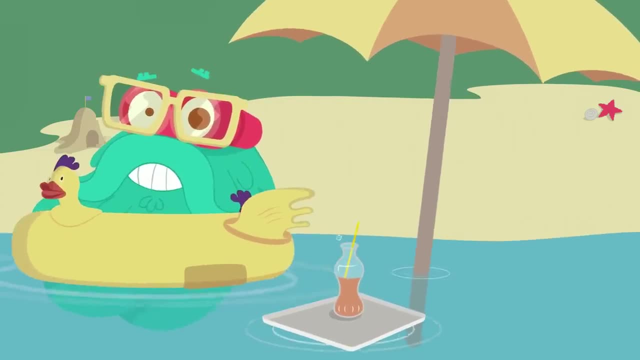 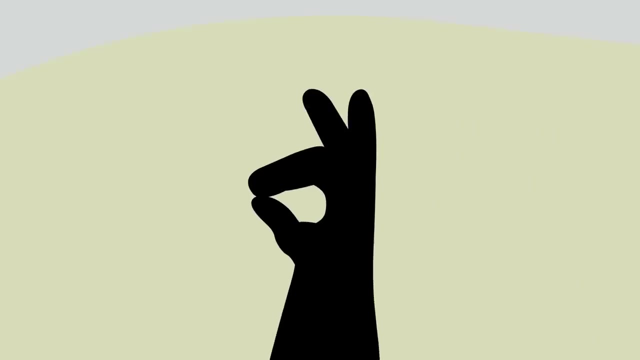 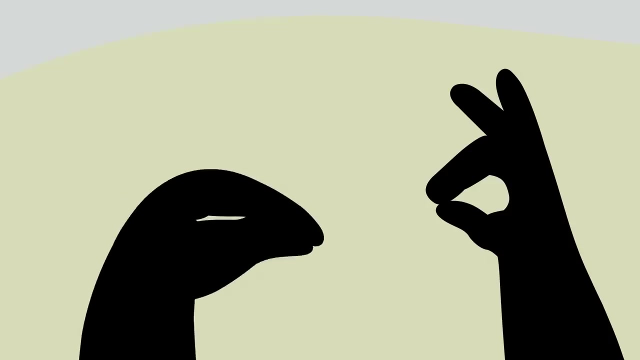 So tune in next time for some more fun facts. Yoohoo, There goes Mr Deer. Oh, And there's Mr Crow. Hey Mr Deer, How do you do? I'm good, What about you? Hey there. 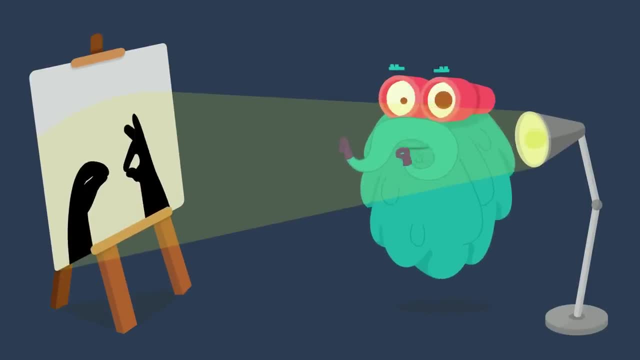 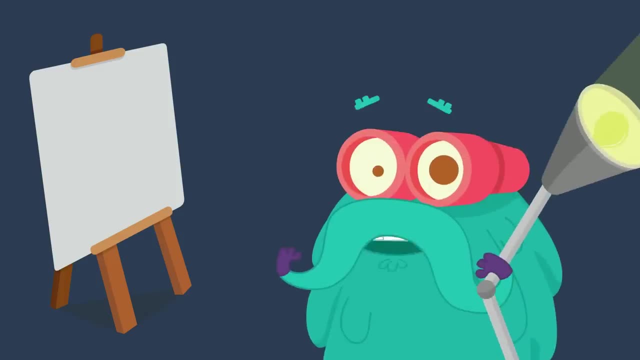 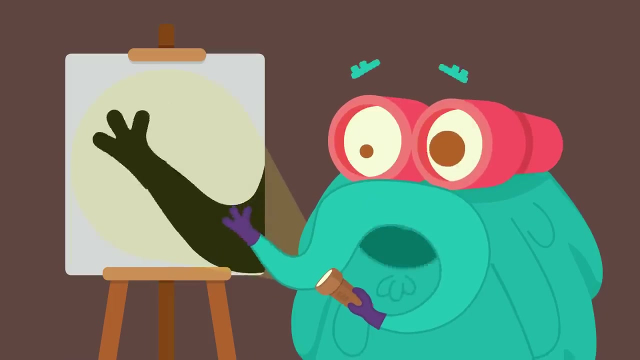 Meet Mr Deer and Mr Crow. No, don't get confused. They are nothing but the shadow of my hands. Come, let me tell you more about shadows. Zoom in. Shadow is nothing but the light that cannot pass through an object. 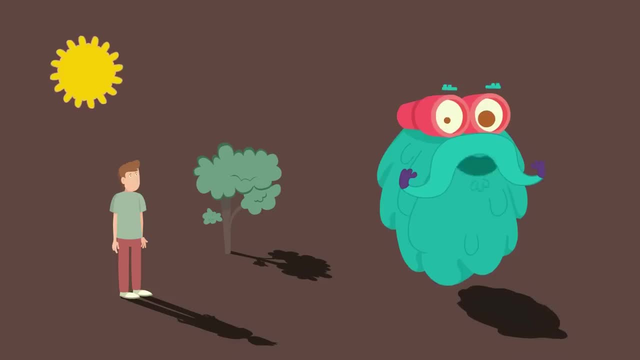 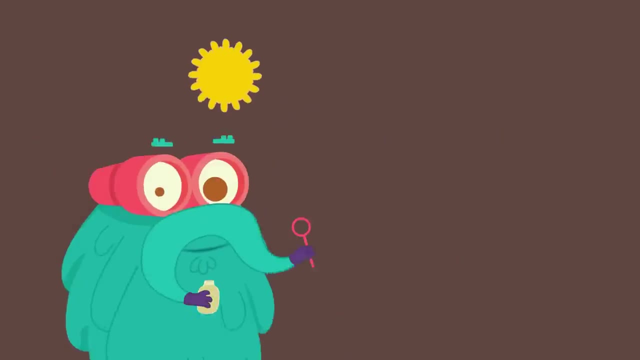 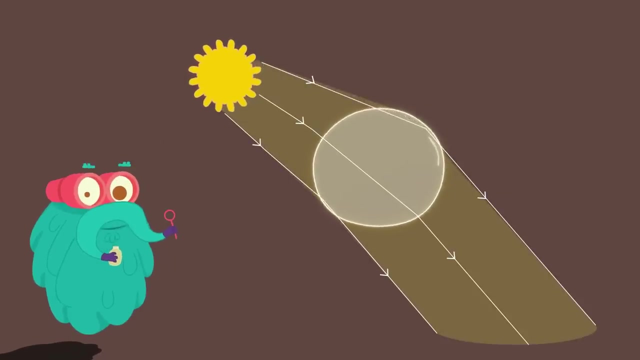 But hey, you can only see shadows of objects that are visible to eyes. For example, a tree will have a shadow, So will you and I, But not air and water, Because light can pass through them. You can have multiple shadows. 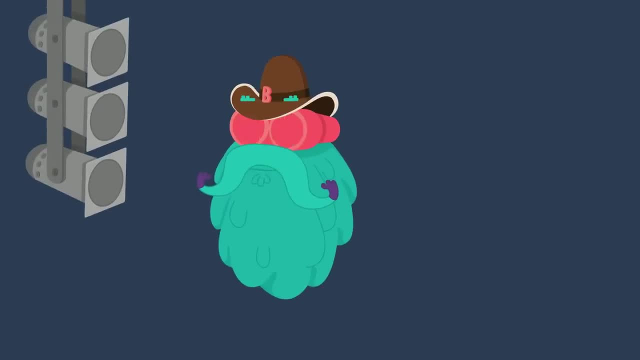 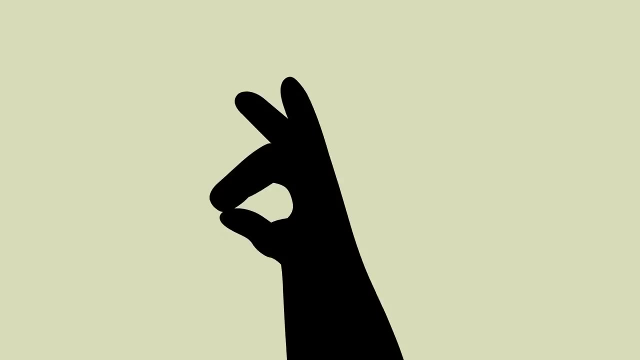 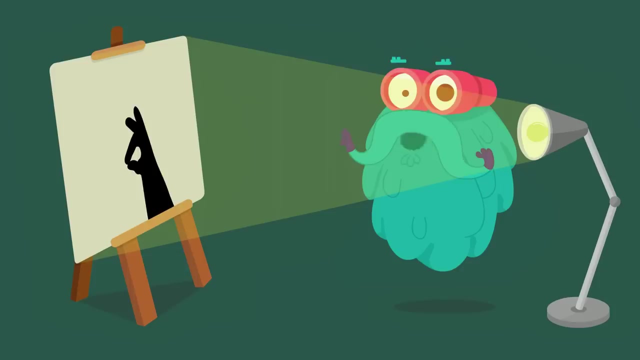 It all depends on the number of light sources. The more the number of lights, the more shadows you will have. Oh, There goes Mr Deer again. Hey, You got to see how Mr Deer changes in size. There's a reason behind it. 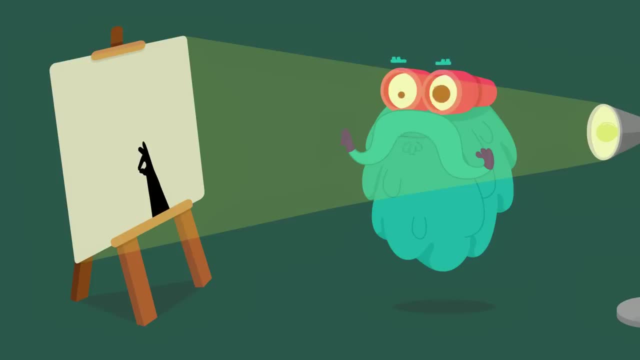 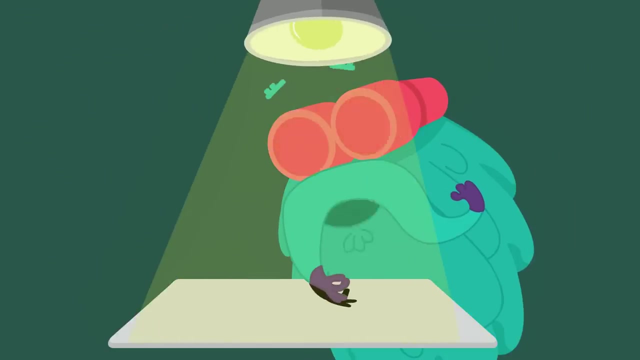 When I move the lights away from my hand, the shadow becomes smaller in size, And when I bring the light source near, the shadow becomes large. When you put the light source just over the object, you get the shortest shadow. Wow, Mr Deer looks so small now. 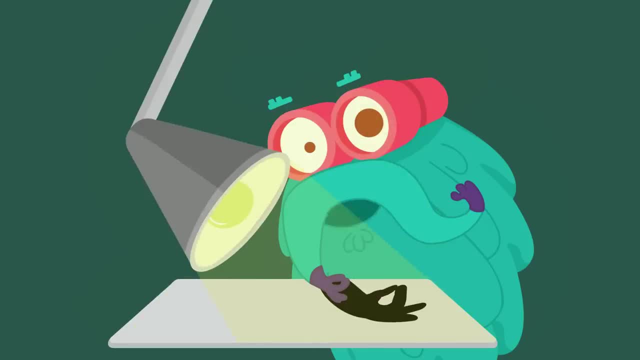 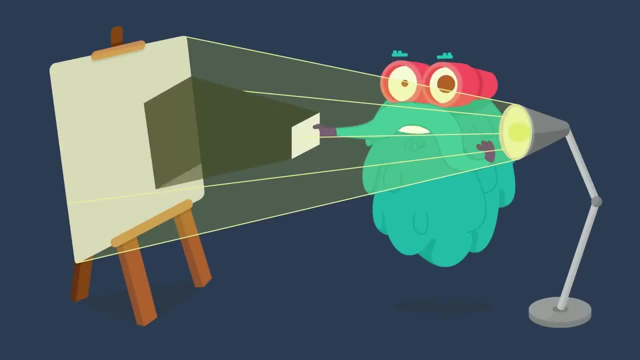 Now you know That the size of a shadow depends on the distance between the light source and the object. It's hard for many to believe that light travels in a straight line. Yes, it's true. Light cannot bend or turn around that object to light up the area behind it. 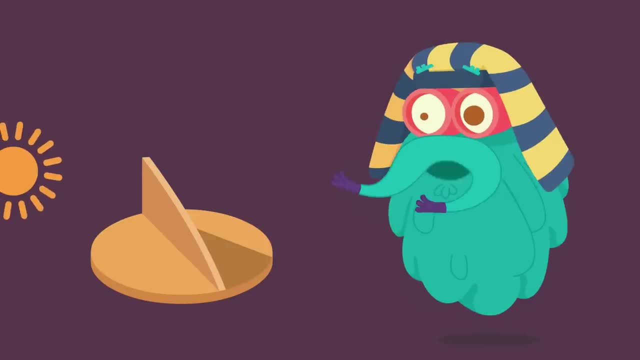 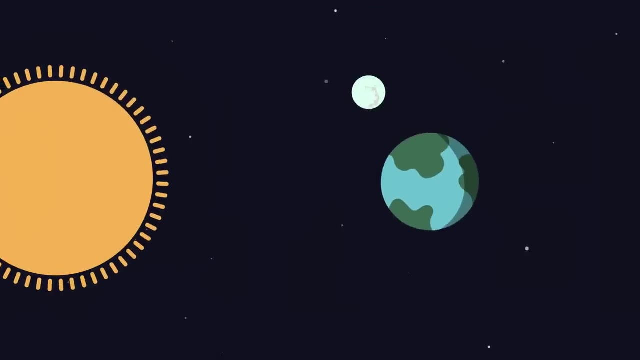 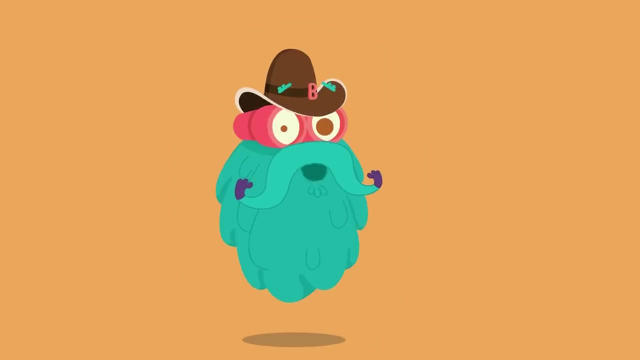 Trivia Time. When there were no clocks, people used to estimate time using the sun clock. A shadow cast by the earth on the moon results in a lunar eclipse, The source of light being the sun. So this is me zooming out. 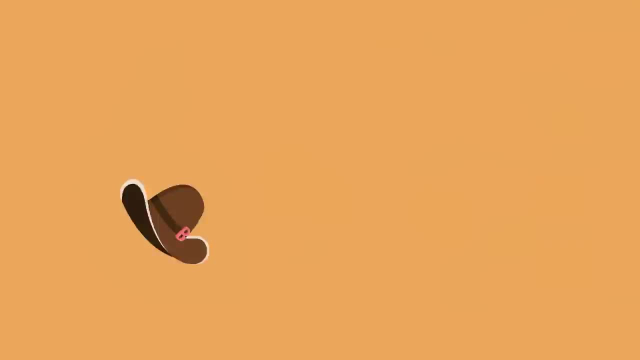 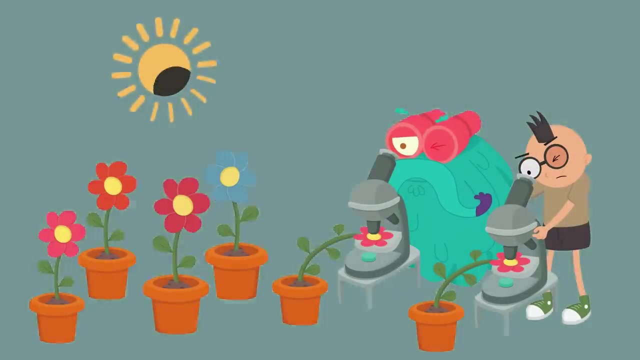 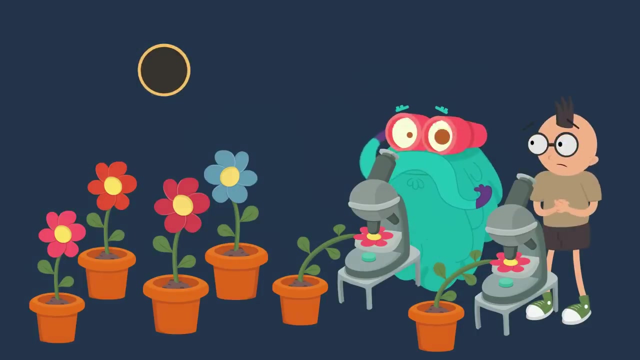 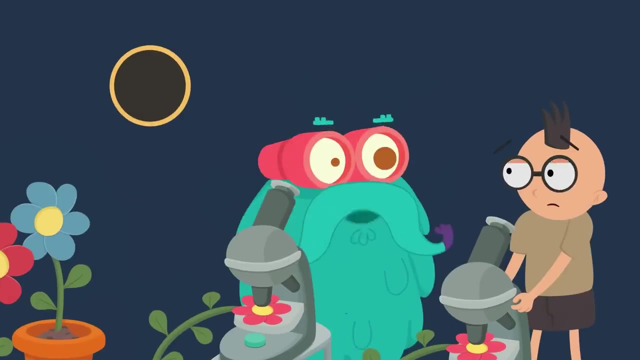 Tune in next time for more fun facts. Hey, Where did the lights go? Is it night already? No, Dr Binox, something just hit the sun. It's scaring me. Oh, don't worry, buddy, This is nothing but the eclipse. 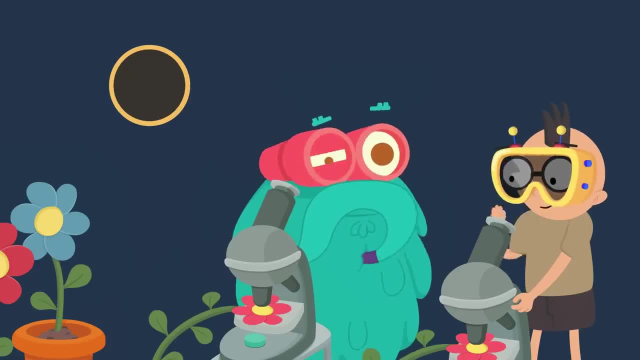 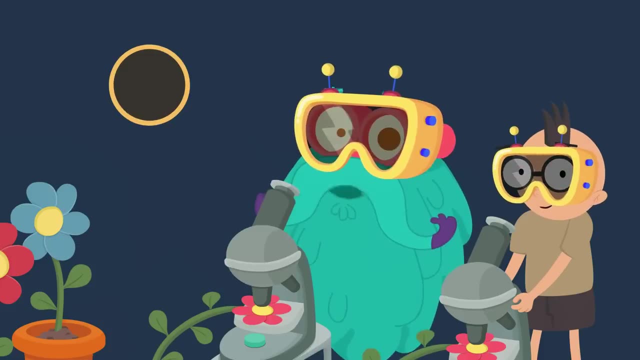 Here, take these glasses. Hello friends, Thanks for passing by. As you can see, the sun's got hidden and it's really dark out here. Do you know what it is? Don't worry, it is nothing but the solar eclipse. 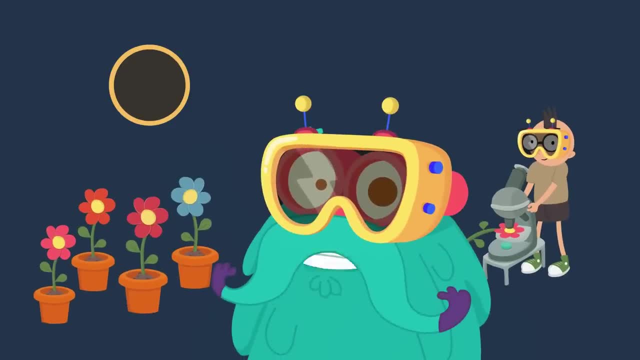 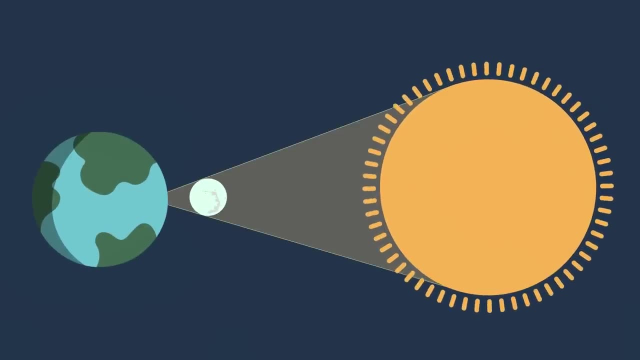 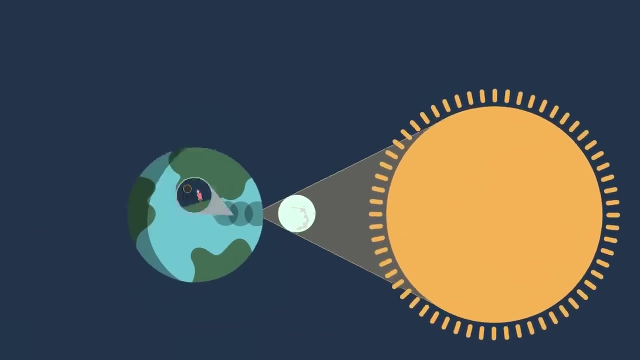 Come. let me tell you something about the solar eclipse today, Zoom in. A solar eclipse occurs when the moon comes in between the earth and the sun, causing a shadow of the moon to fall on certain portions of the earth. From these locations, it appears as if the sun has gone dark. 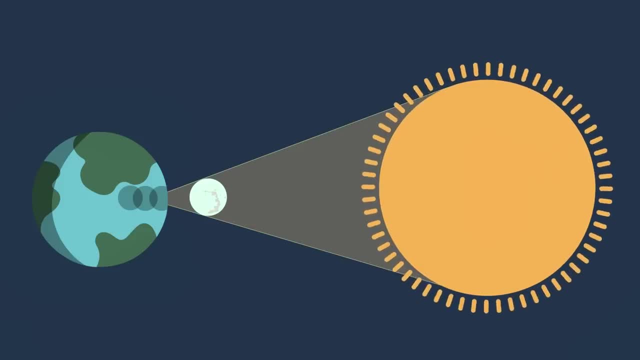 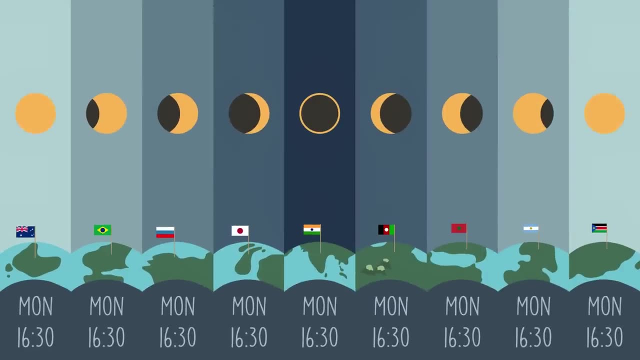 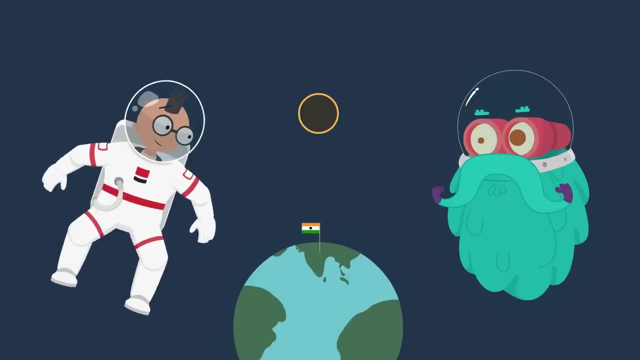 Since the moon is very small in front of the sun, it only blocks a part of it. Hence, a solar eclipse cannot be seen from every part of the earth, but only from the locations where the shadow of the moon falls. So, buddy, no reason to get scared now, is it? 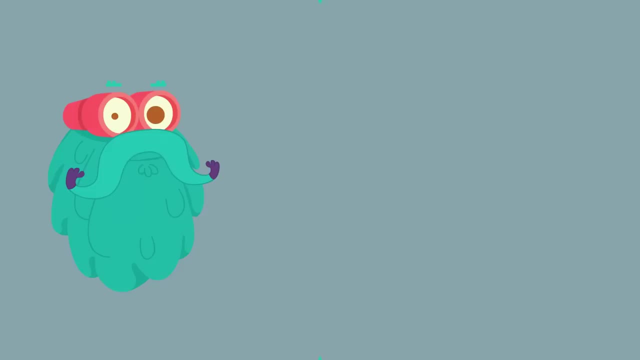 No, Dr Binox, not at all. The three major parts during a solar eclipse are Umbra, Antumbra and Penumbra. The umbra is the portion of the moon's shadow where the moon completely covers the sun. This is when the total solar eclipse occurs, where you cannot see the sun at all. 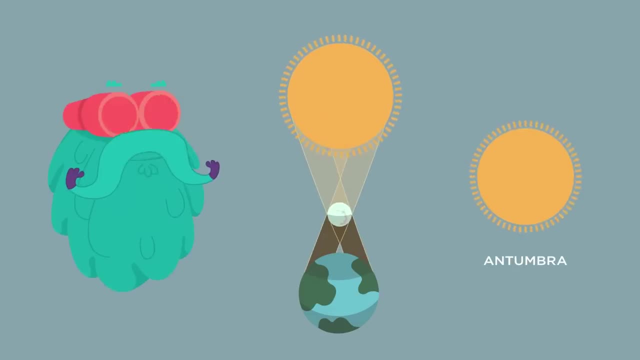 Antumbra is the area beyond the umbra. Here the moon is completely in front of the sun, but doesn't cover the entire sun. The outline of the sun can be seen around the shadow of the moon, And that is when you see the annular solar eclipse. 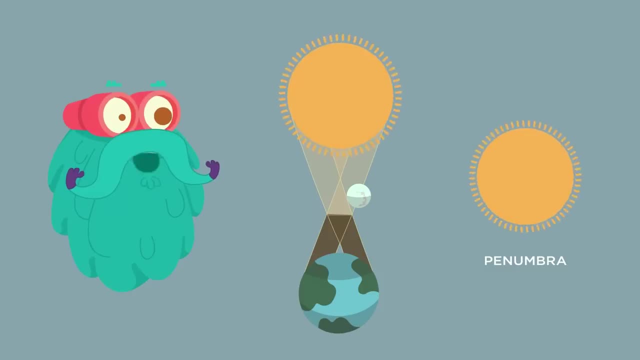 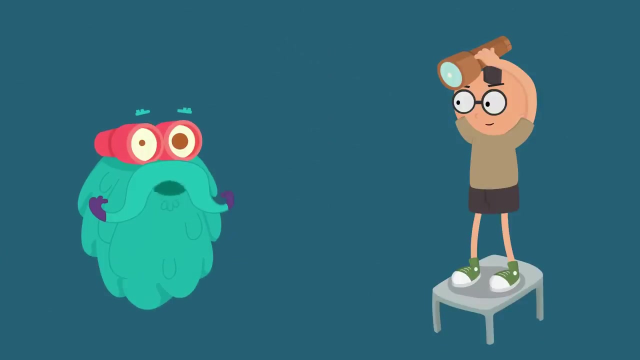 Penumbra is the area of the shadow, where only a portion of the moon is in front of the sun. This is when the partial solar eclipse occurs and lets you see only a part of the sun. You could see how the solar eclipse works in your homes. 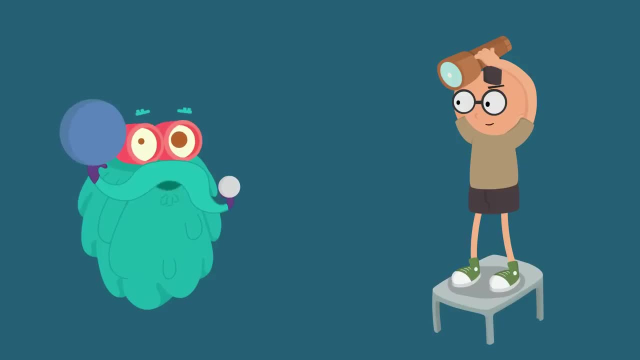 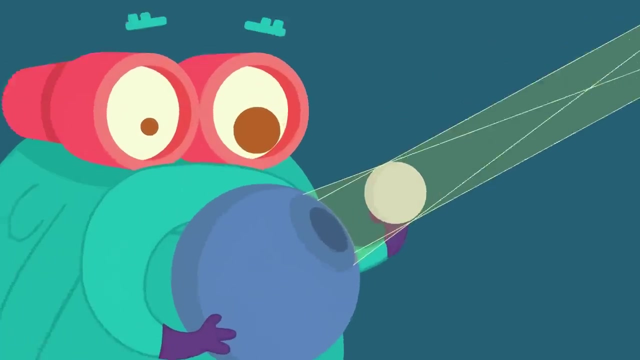 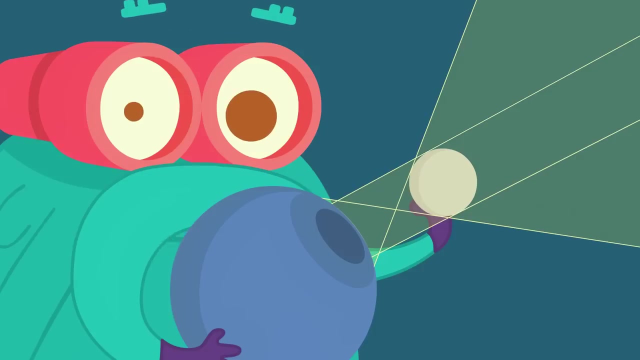 Take these two balls: The bigger blue ball is the earth and the smaller white ball will represent the moon. Place them like this and light up the torch. The torch will be our sun There. there, You just got a homemade solar eclipse. Amazing, isn't it? 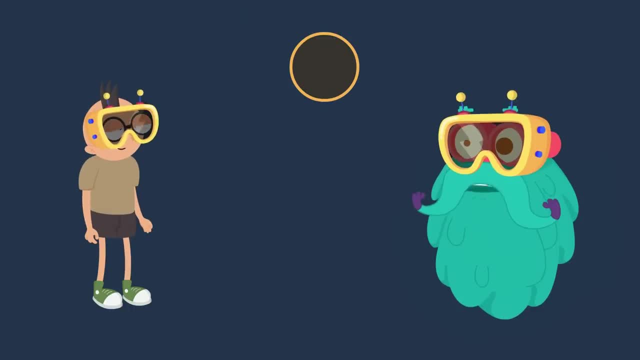 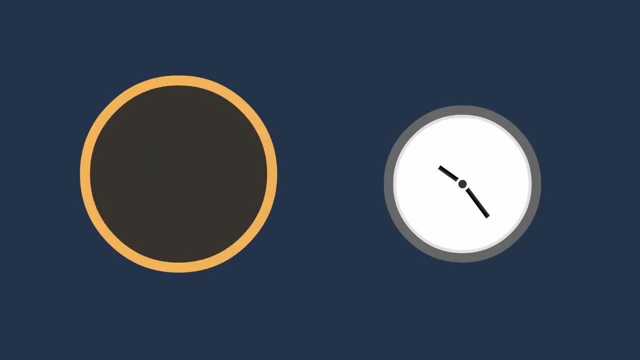 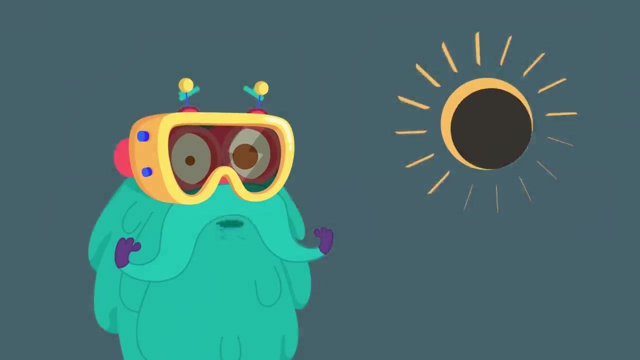 Trivia time. One should never watch the solar eclipse with bare eyes because of the harmful UV rays. The longest a total solar eclipse can last is seven and a half minutes, So now, if day suddenly turns into night, you would know it is the solar eclipse. 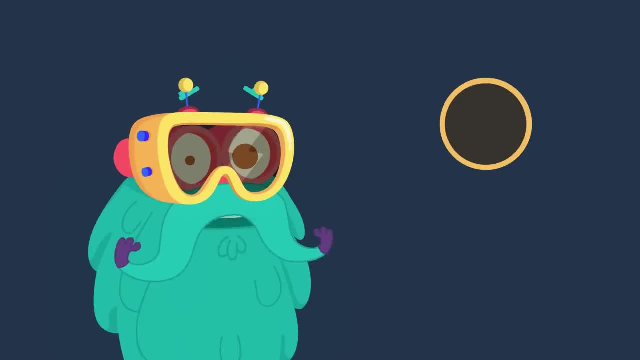 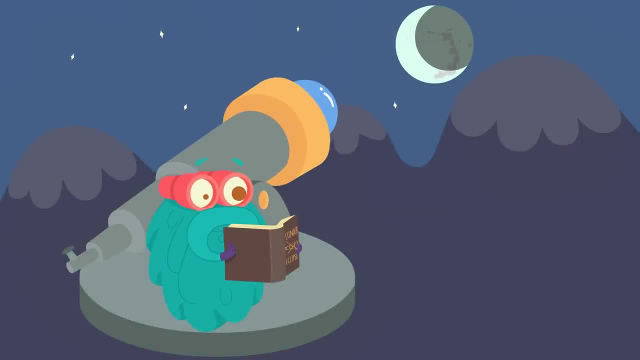 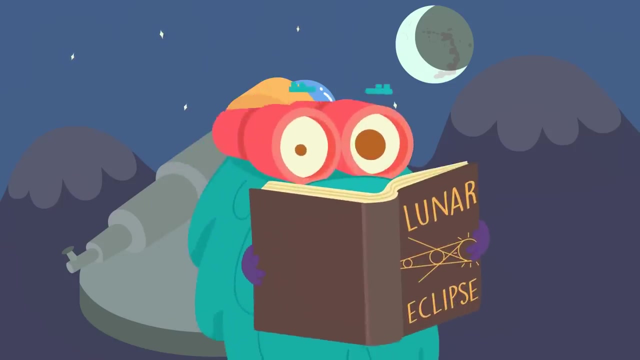 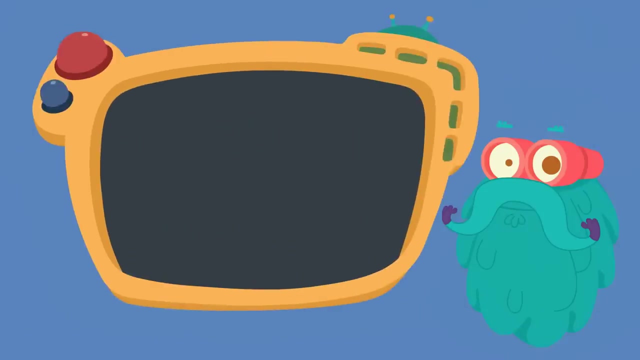 This is me zooming out. Tune in next time for more fun facts. Hey Care to look at what I am reading. I am reading about the lunar eclipse. Let's see what it is. Zoom in. A lunar eclipse happens when the earth moves between the sun and the moon. 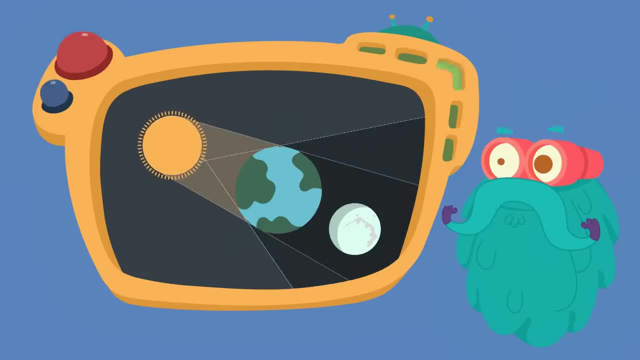 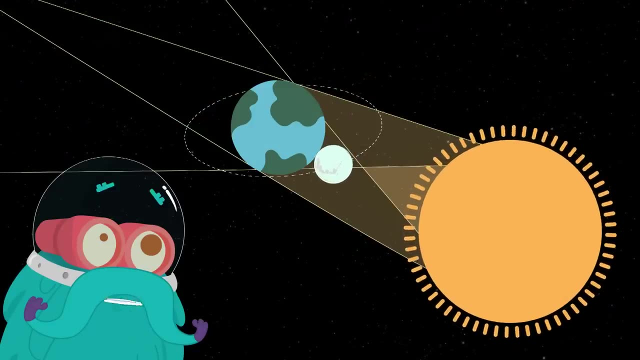 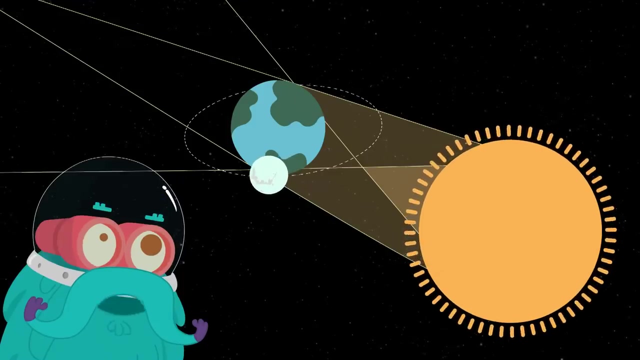 Blocking the sun's light from reaching the moon. Come, let's go to space and see how the lunar eclipse occurs. You see them: The sun, the earth and the moon. Look how the moon is slowly passing from the penumbra to the umbra. 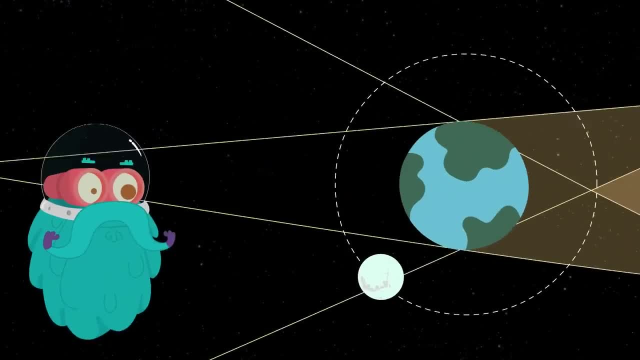 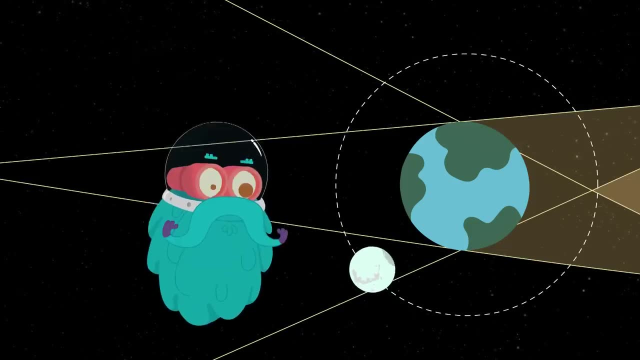 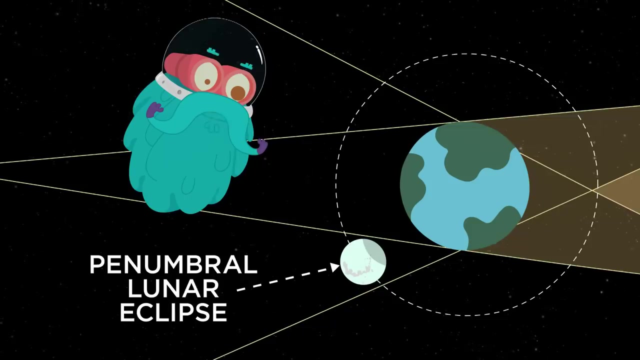 Hey, Stop, Stop. This is the penumbra, the region beyond the umbra. Okay, moon. When the moon travels to the penumbra, we see a penumbral lunar eclipse where the moon is faintly visible to us. 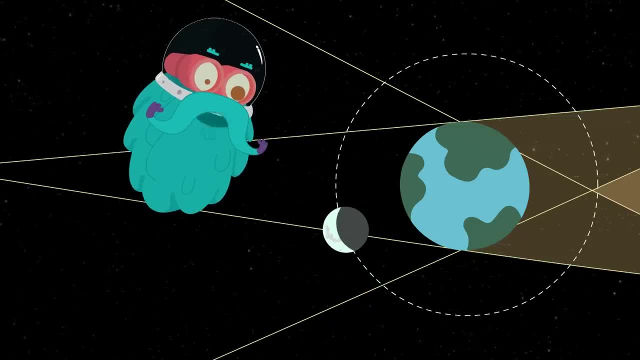 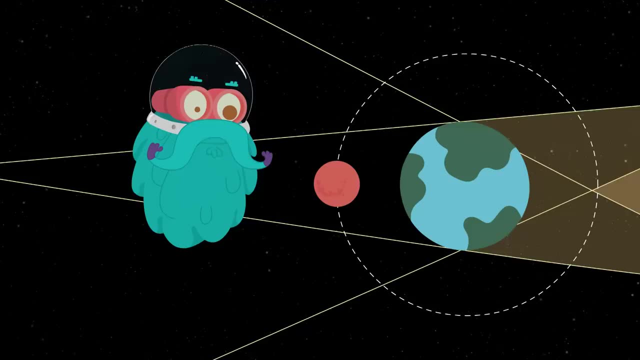 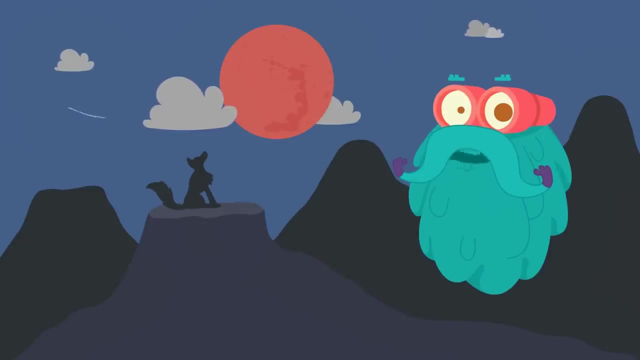 When the part of the moon is in the penumbra and a part of it is in the umbra, we see a partial lunar eclipse, And when the moon travels to the umbra, we see a total lunar eclipse. There are times when the moon appears to be red. 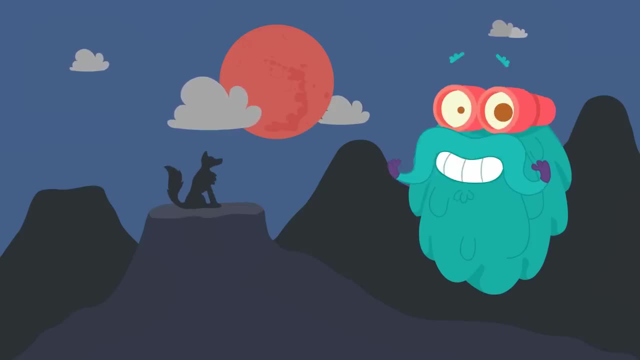 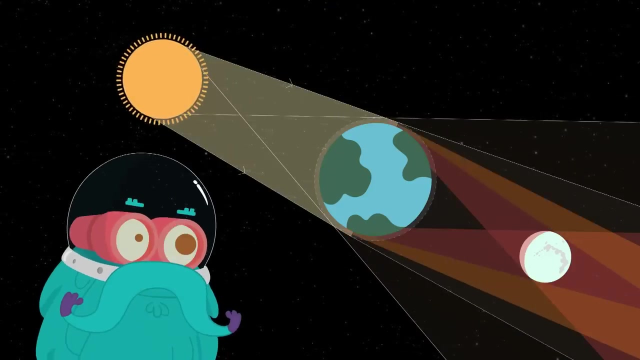 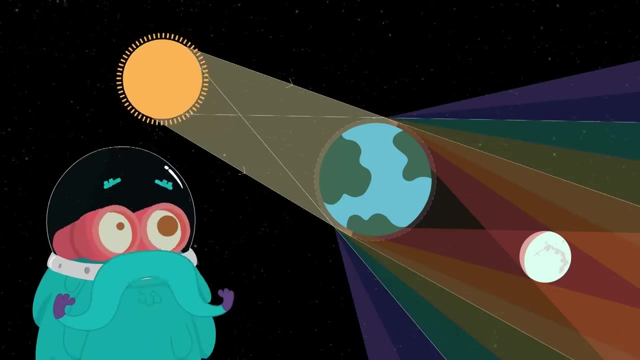 Oh, don't be scared, I'll tell you how that happens. As we all know, the rays of the sun are made up of red, orange, yellow, green, blue, indigo and violet. When the sun rays hit the atmosphere of the earth, most of the colours get scattered away. 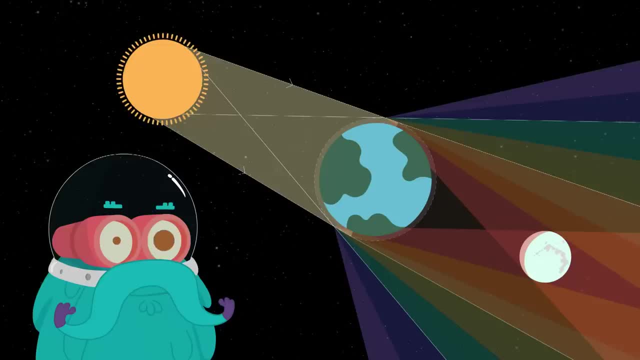 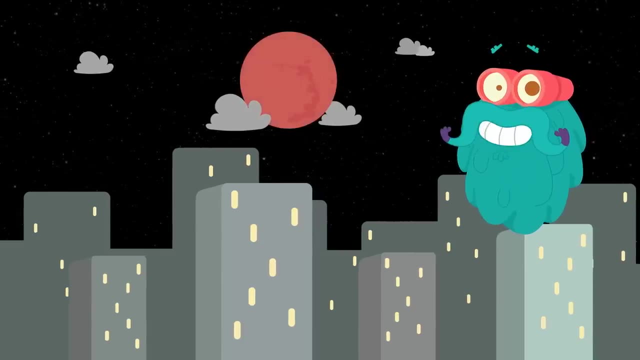 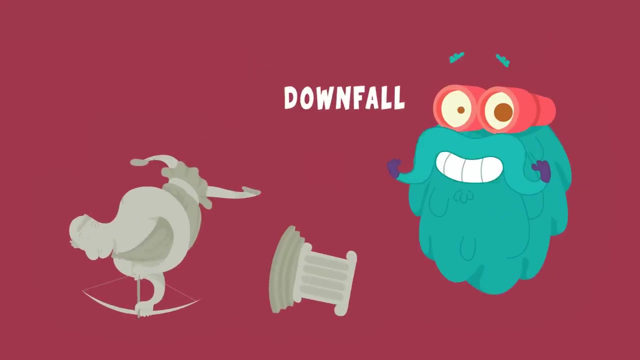 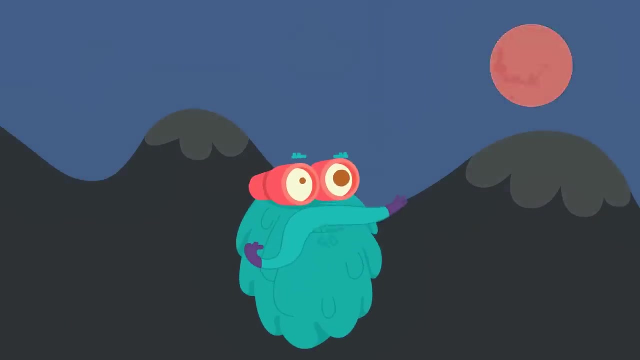 And the colour red remains, Due to which we see a red or a blood moon during a total lunar eclipse. Trivia time. The word eclipse in Greek means downfall. A solar eclipse always takes place about two weeks before or after a lunar eclipse. 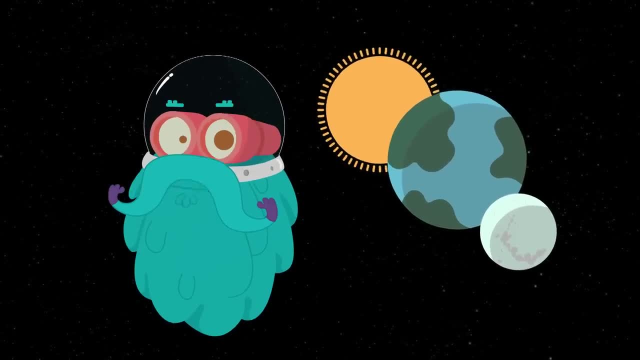 So now you know quite a lot about the lunar eclipse, Don't you? This is me zooming out. Tune in next time for more fun facts.